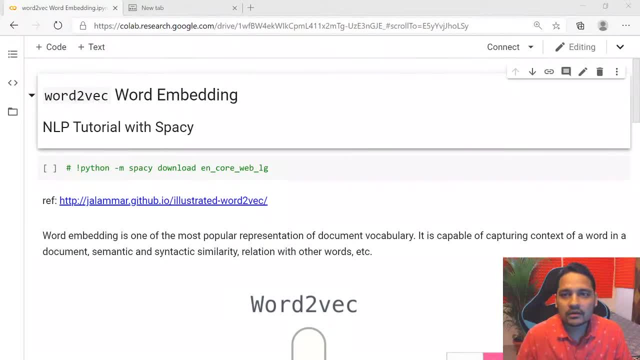 it all right. so it's is that there is a problem. all right says that YouTube. YouTube is not receiving here enough video to maintain it's a smooth streaming. I'm not sure, guys, if you are there and if you are able to, if you are able to see me, please let me know. all right, good union, good union, how are you? 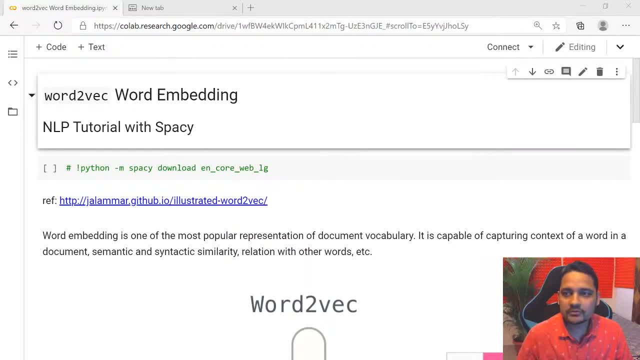 Hassan. all right. so it's ill to all of you. all right. so for good union, good union, providing good uni, all right. so we have liked. today we are going to talk about what to vector, what embedding. I and this NLP tutorial is going to be with a specie and we will be coding in the 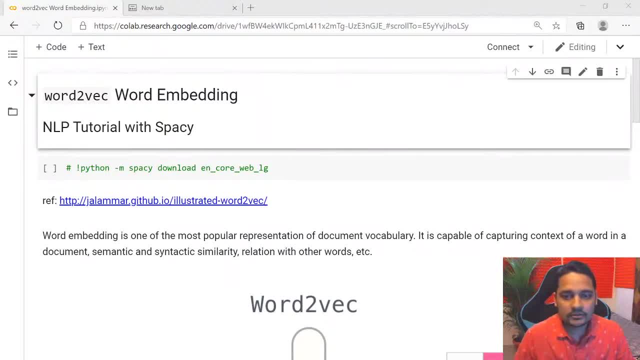 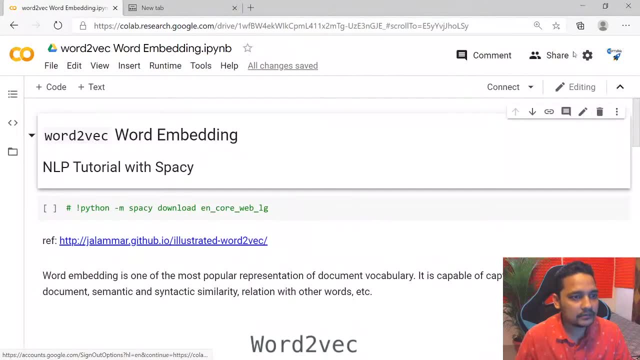 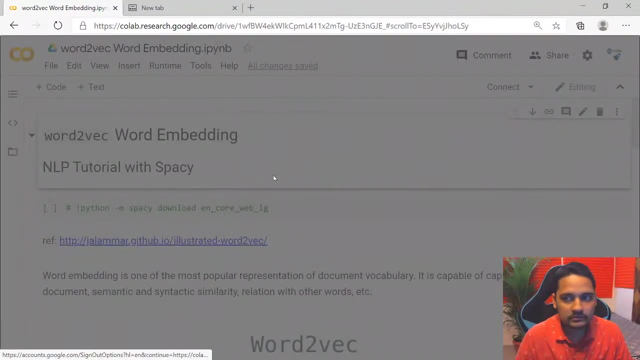 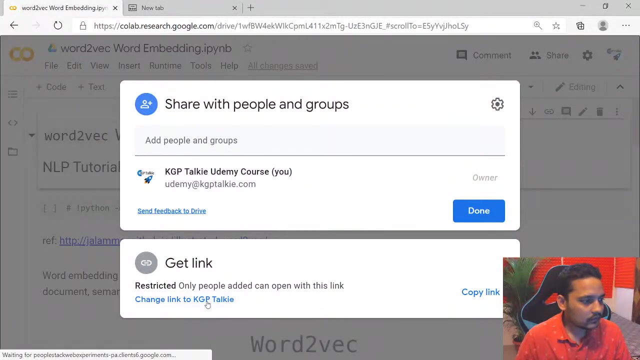 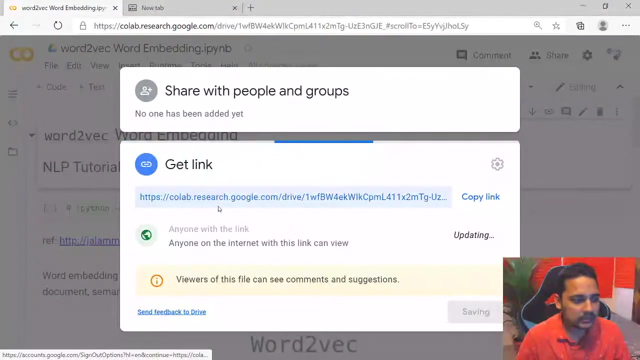 Python there. all right, so the first of all, let me share this notebook so that we can share this notebook from here, perhaps so that you can also get, so that you can also get started with these, this notebook, all right, okay, let me make it. anyone with the link. 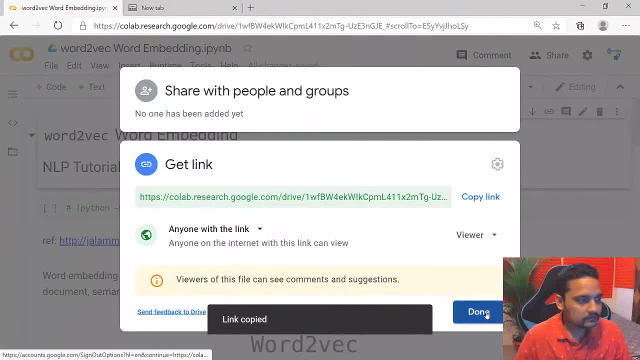 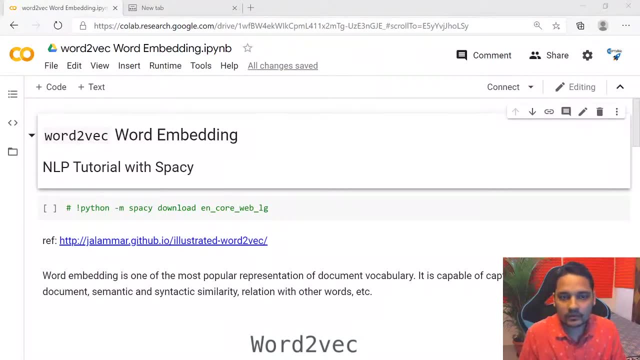 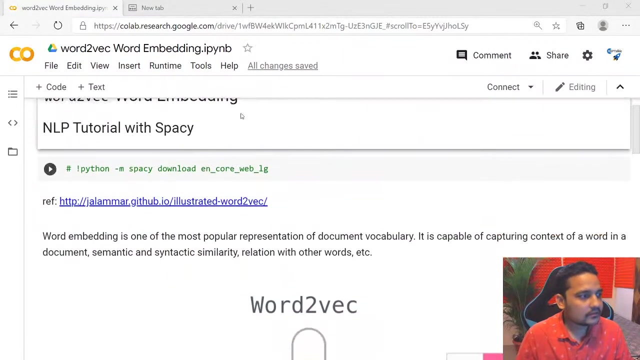 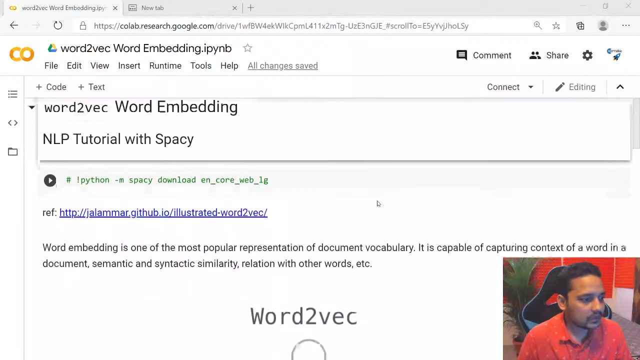 all right, superb, let me paste it here. let me paste it here, let me paste it here, all right. so currently you should be having a notebook, a live notebook, with you, all right. so we are going to talk about here, word to vector, word embedding, and here i have taken few of the images from this blog. 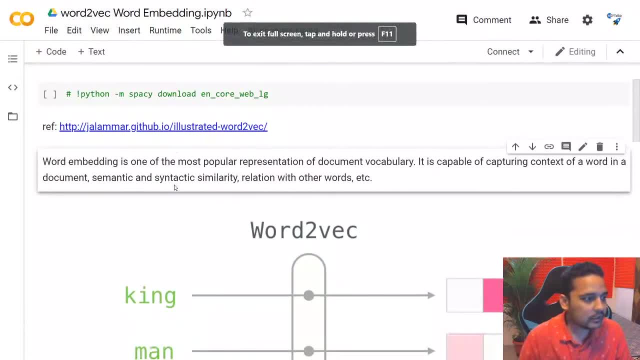 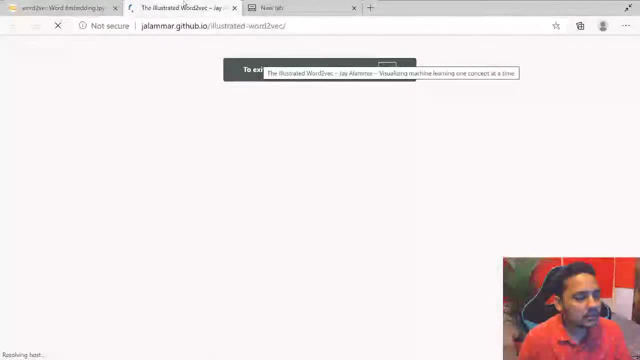 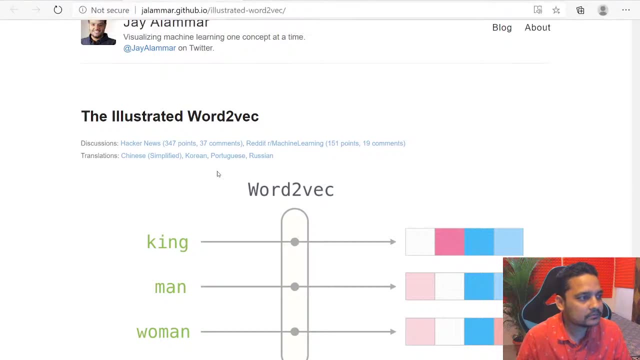 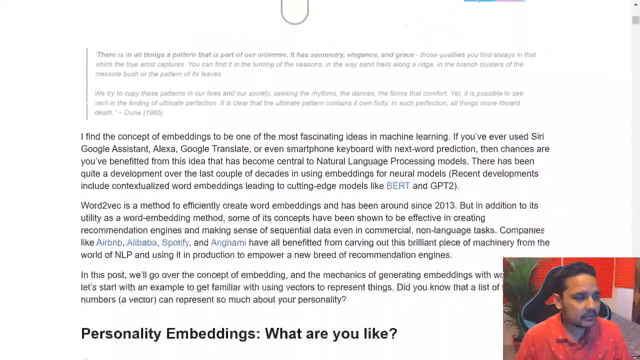 all right there. we have a very good blog here, so it is available at github and, moreover, if you want to have here a very basic knowledge of word to vector, you can definitely come to here and you can learn about it. but it's kind of very you know the ground and very basic and the coding is not available here. but if you want to learn, 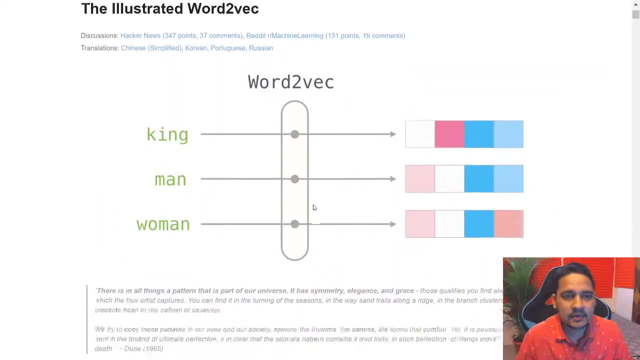 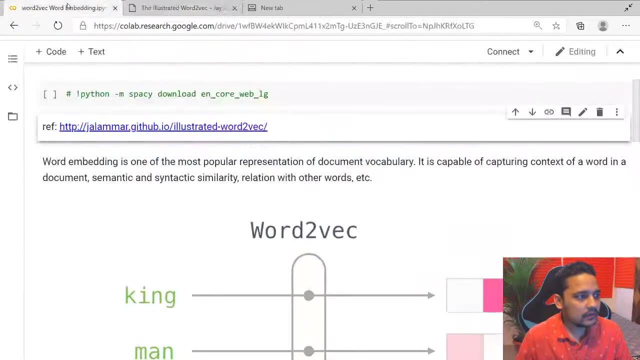 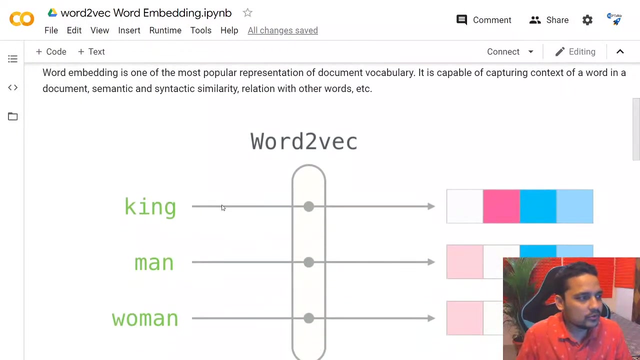 about the theory, part of word to vector, then these things are available here. all right, so, and it's a very good blog, so i have taken few images, so let's go ahead. come back to our notebook here, word to vector notebook. so in this notebook, you see, there the first of all you have to. 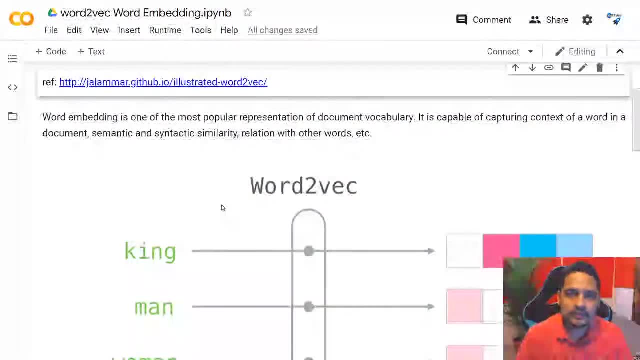 understand that. what is word to vector, word embedding, and why do we need this word? word embedding: see, the computer cannot understand text data. we have to have something which can represent our text data in the numerical data. like we work in our image processing, their image get converted into a numpy area or a numerical data. similarly, we have to make something that so that 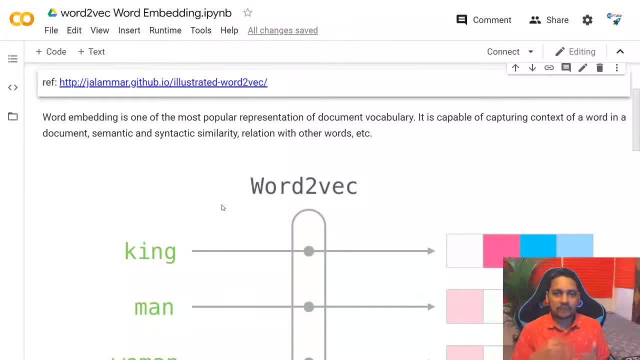 we can convert our text data in a numerical representation. all right, the way we convert our text data in numerical representation, that is known as word to vector, word embedding, and this is the just one way. there are many more other ways in which we convert our text data in. 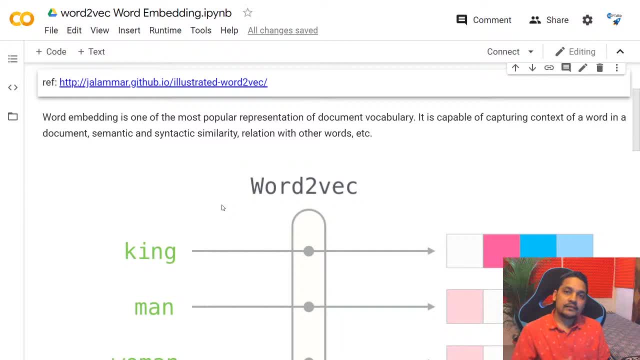 numerical data, which is known as a vector, like there is a glove vector. a glove vector is a global vector representation. all right, and apart from that we have their continuous bag of word, a term, frequency. word counts otherwise. we have another very famous tf-idf word embedding that is the tf-idf term frequency, and then multiplied by inverse document. 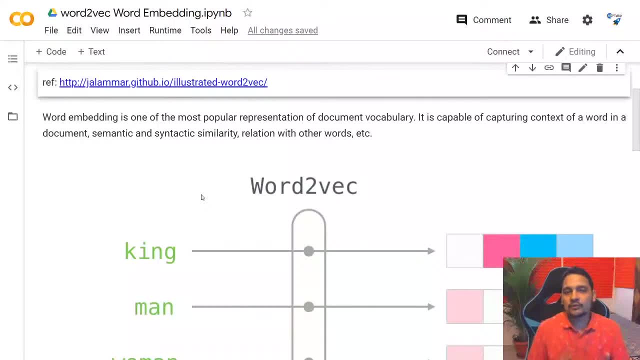 all right. so those are the ways to convert our text data in a numerical representation and the same thing we are doing here. we are converting our text data in a numerical representation and the way we convert our text data in numerical representation. those depends on how good algorithm we are applying in those conversation and if you apply a good algorithm. 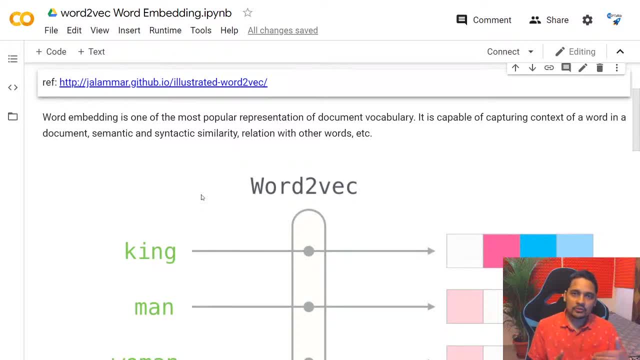 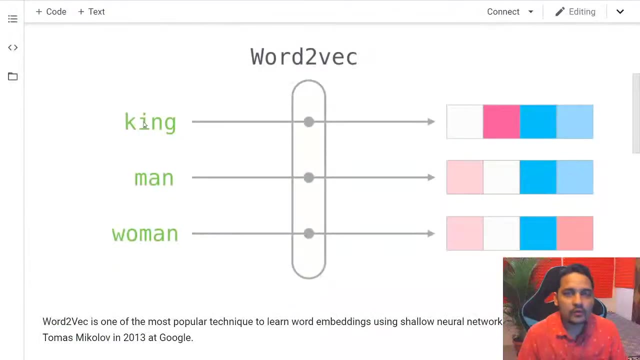 then definitely you will get a get, you will get a good accuracy. all right, thanks, romeo mendes. thank you all right. so to understand this word two vector, you can understand with this figure that let's say you have these two words: king, man, and then you have their woman. 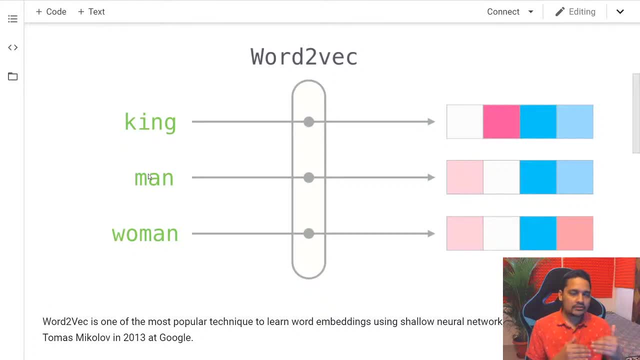 king, man and woman in, though, in these three words. so the king is much more correlated with man instead of this woman. all right, so king and man will come into a same category, and king and woman will not come into a same category. i mean, the similarity will be much more. 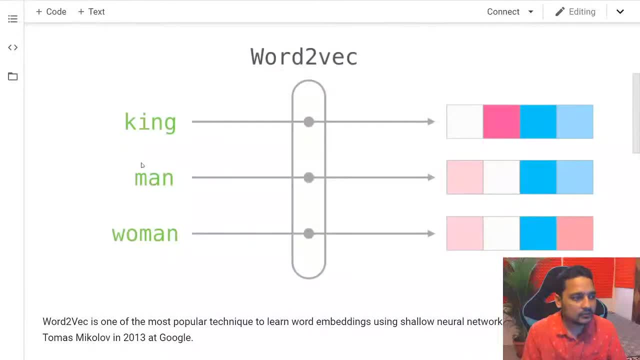 you know, high in between the king and man, instead of this king and woman, but the similarity between this man and woman will be high instead of this. uh, you know king and woman. so the moreover, how it is happening. it is happening that king and man, those are falling into a same category, all right, and this man and women are also falling. 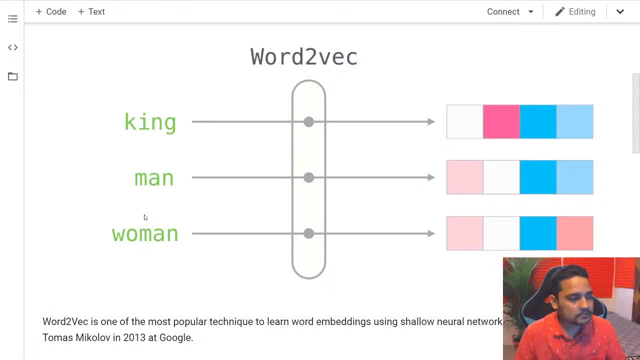 in the same category. so so so you know the similarity in word, two vector will be high for these combination of words. two vectors will be high for these combination of words, and you can also understand with these representation that if you notice that here these two are more similar than this one and this one, all right. so if you, 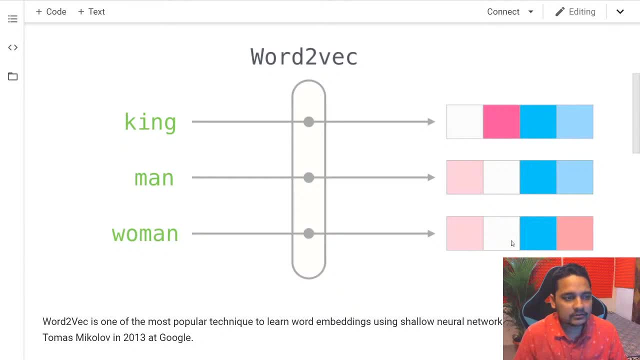 if you talk about that, these are the vector representation. so by seeing this, the by seeing just these vector representation, you can find out that this king and man, these vectors, are much more similar than this king and woman, all right, and this man and women are also similar, all right. so 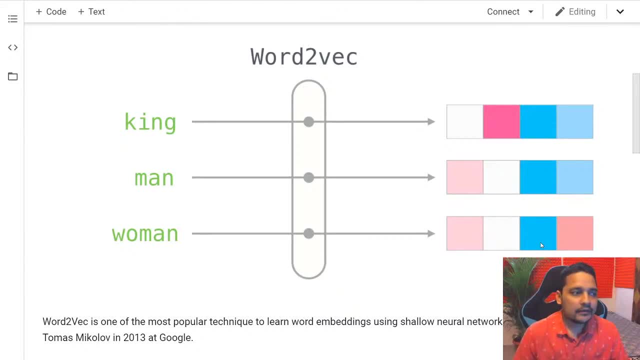 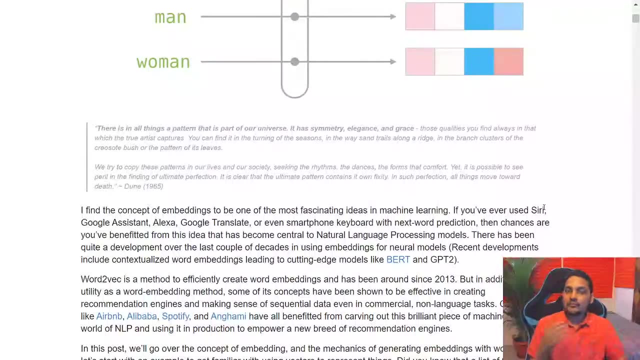 that is how we calculate the word to vector. now, if you read in this blog, so this blog says that how you can convert your text data into a vector from a scratch. all right, but many times we don't need to work from a scratch and and we already have all, uh, trained to do the work from scratch. 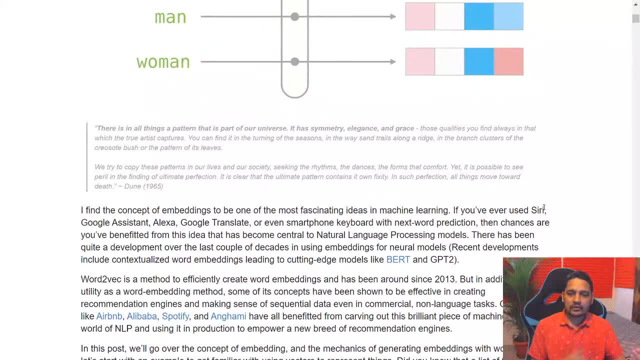 algorithm. all right, so there are already pre-trained algorithm available. all right, so we already have pre-trained algorithm available with a spacy, so we'll be using those algorithm with a spacy, all right? yes, romeo, i'll try to make one video- chatbot video. so i'm 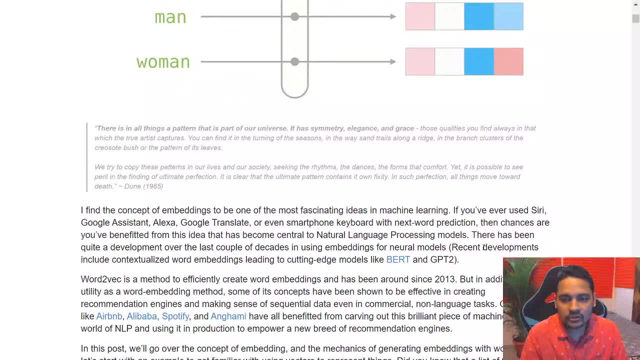 currently preparing a lesson on udemy. so, on udemy, currently i'm covering with the nlp basic, but later i'll also try to make one more course there with advanced nlp, which will be basically based on the chatbots and transformers like bert or robert or gpt and elmo models, all right. so 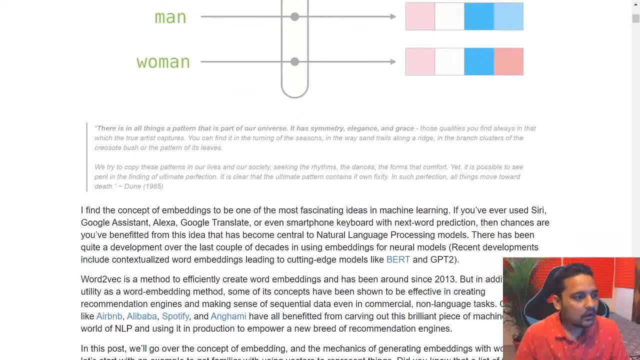 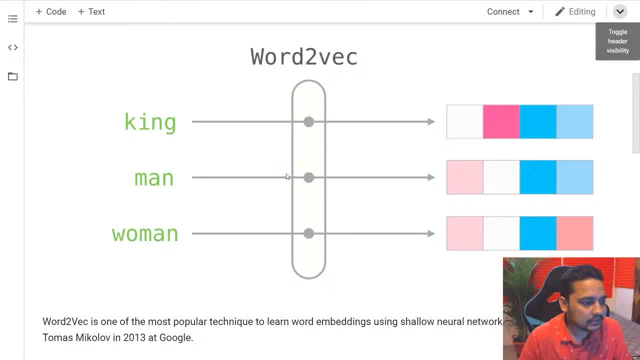 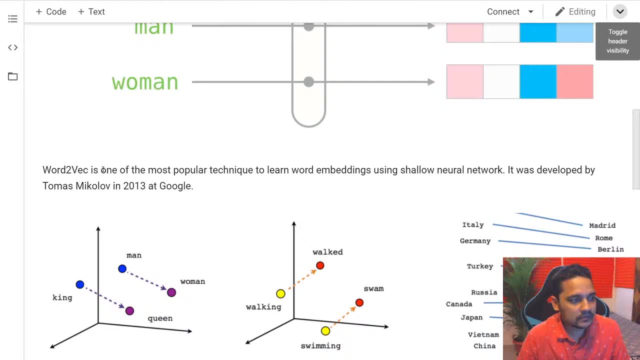 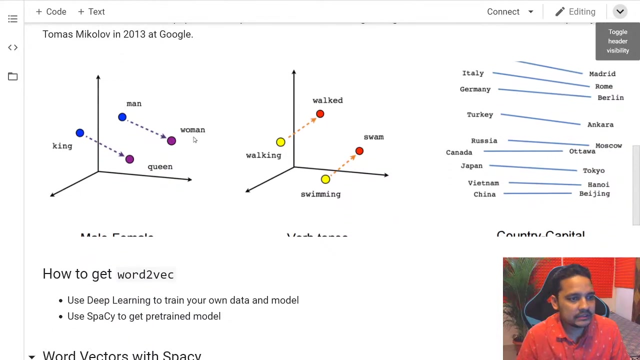 those are the transformer models. all right, so that is how you can convert your text data into a numerical representation, and this word to vector: you representation. this was a algorithm. this was developed by google in 2013. all right, and here is another example which- uh, you know, this shows almost. 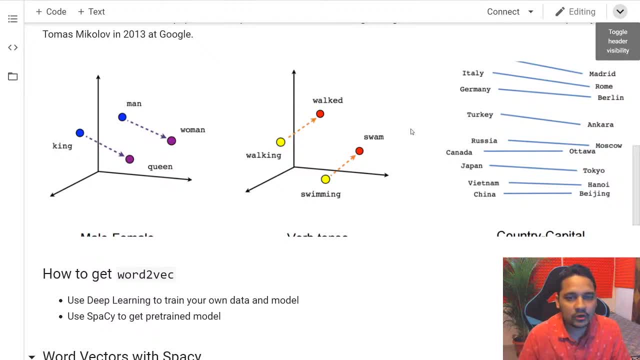 the same concept which we talked earlier, like, uh, this man and king are, you know, falling in a kind of same category, are in same dimension, and then woman and queen are also falling here in a same category. there, all right, and there, uh, in the same way. you can also understand, here we have 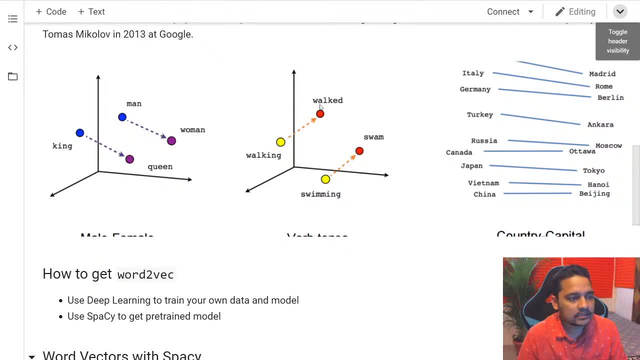 walking and walked, all right. so there is a past participle. so this past participle for a swimming, there is past participle for this verb is also swim, all right. so the direction of a similar kind of words are same in the word to vector representation: all right, and the same thing is. 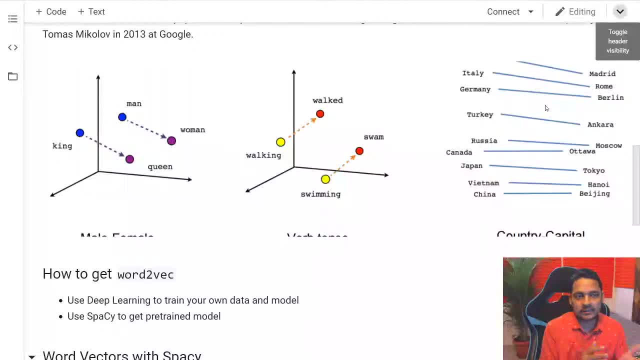 here, which will tells you that, says you should stick to, and does which. then you are here with the number of answers in your head and the other thing is: uh, as you're talking, definitely you hear it. so that's another way of past participle, so it also shows: 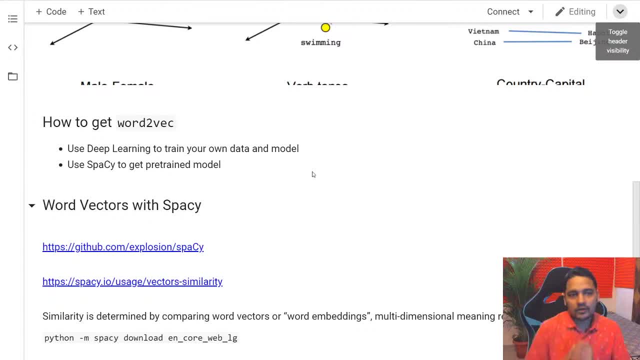 that, uh, but for example, like there is a, this person in a mirage, so if you do a or, let's say, you learn fiction call夫, so there is a constant. thus you, as you require the cambiating and behaviour, them from a scratch. otherwise, what you can do, you can use pre-trained model, a pre-trained vector. 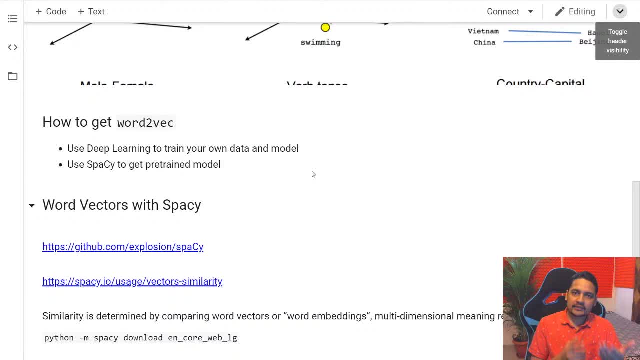 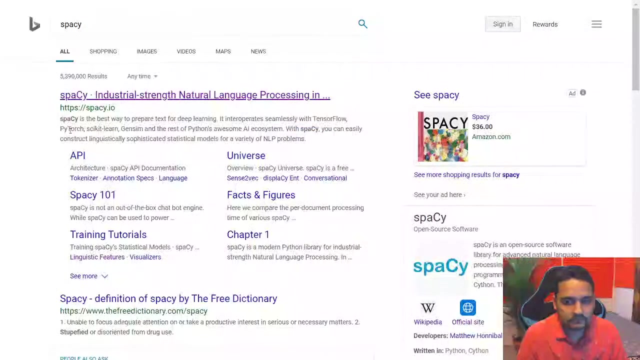 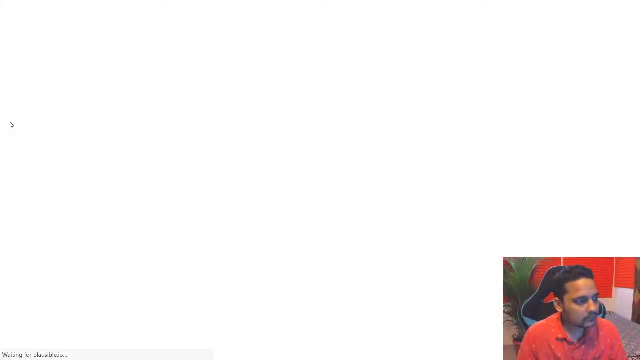 model which are already available, and then we can filter that's mean vector from the library and then we can utilize it. all right, so we'll be getting it from a spacy, so to know more about the spacy here, so let's go ahead and type there a spacy, all right? all right, so there you have here. 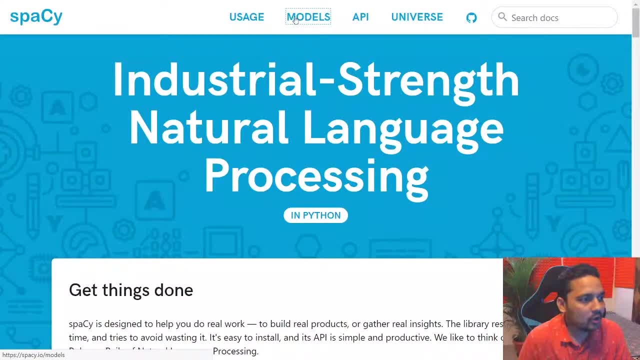 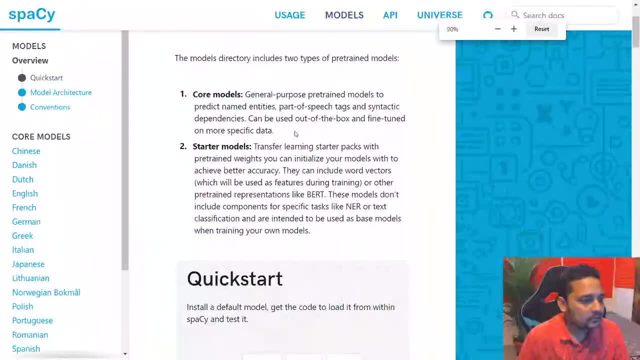 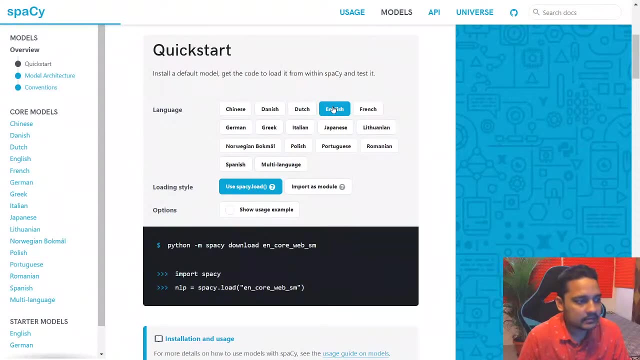 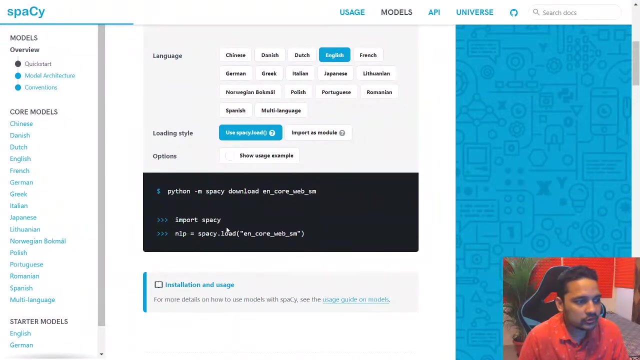 you can come, I think, in the models you should have here, all right. so in models we have here, a model says that how we can utilize this spacy in our application. let's see if we select here english, all right, and we want to use it like this. use spacyload so you can use it like this one. 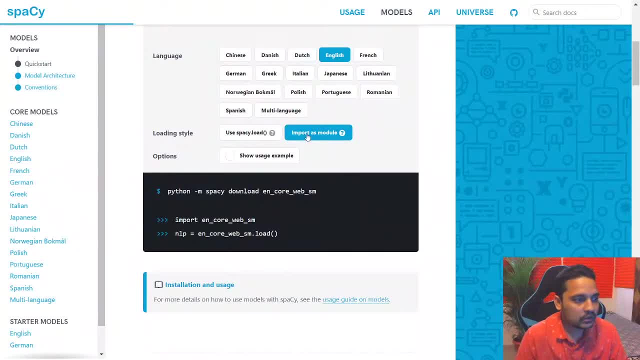 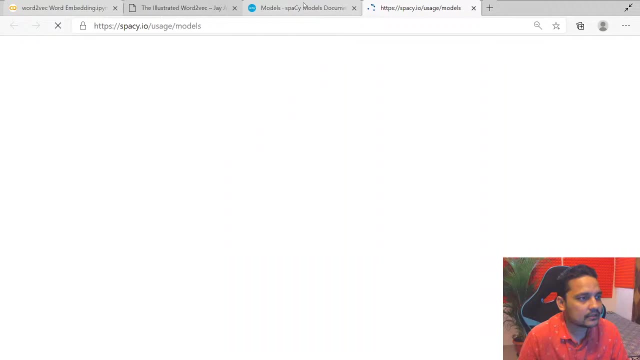 otherwise you can do import as a module. all right, then you can import it. something like this one, and there is, if you select here, so as example you will get. otherwise you can also open here so that you can know about its installation. so installation is pretty much simple. this one says: 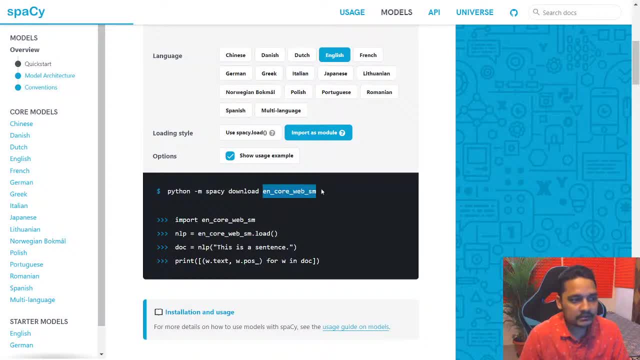 that how we download pre-trained vectors and pre-trained models and apart from that, we will be also downloading here a spacy. all right, let's go ahead. come back to our notebook. so in this notebook we have a spacy and we will be downloading here a spacy and we will be downloading here a. 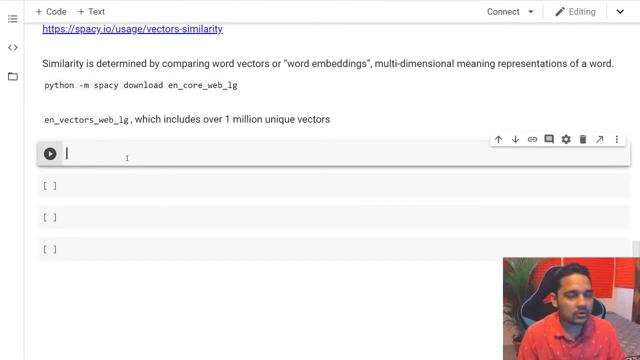 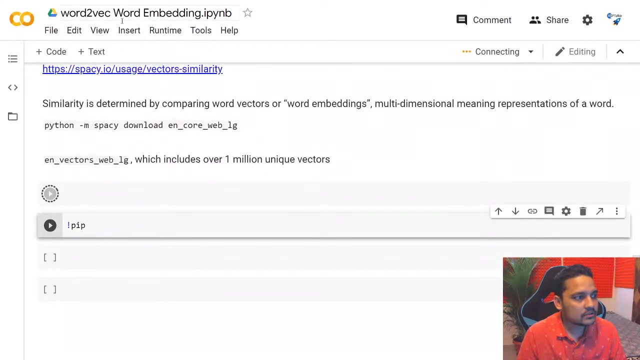 first we will be installing a spacy and then we will be installing here the this model- all right, wave large model, because we need here word to vector. all right, so you can, you can do it here. so do remember, this is this one is google colab, in which we are working currently, so we have here. 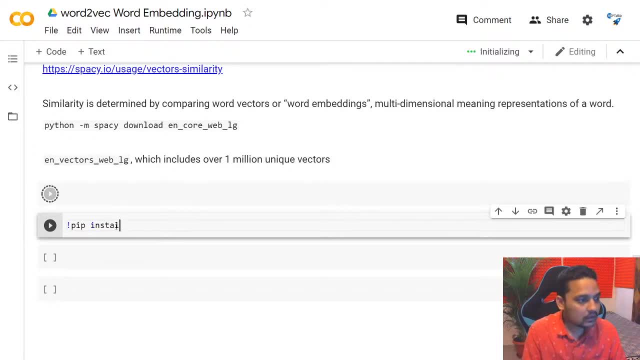 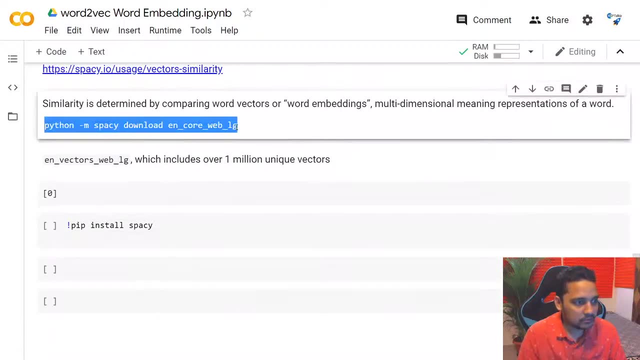 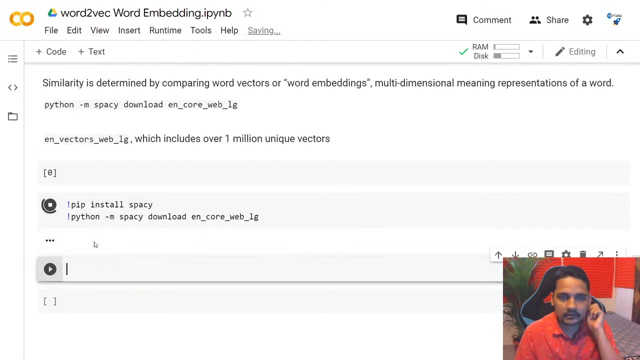 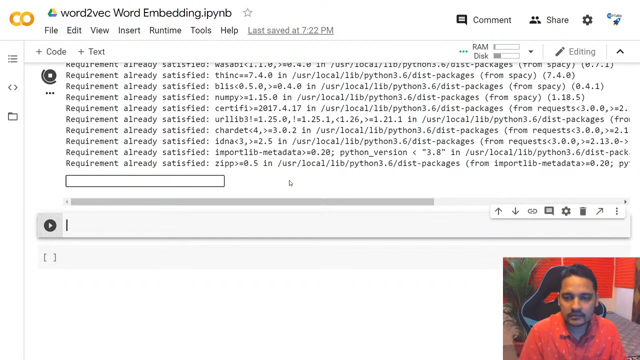 a pip and then install spacy, and thereafter we are also going to install here a large model of a spacy. we can do it with the exclamation mark there. let's go ahead and run it, so it might take a while to install it in meantime. if you have, guys, any question you can ask. all right, and thanks. 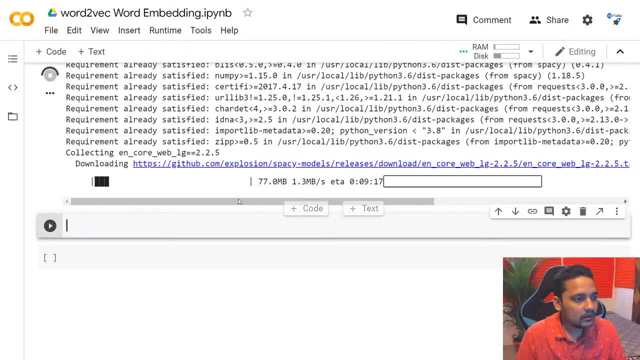 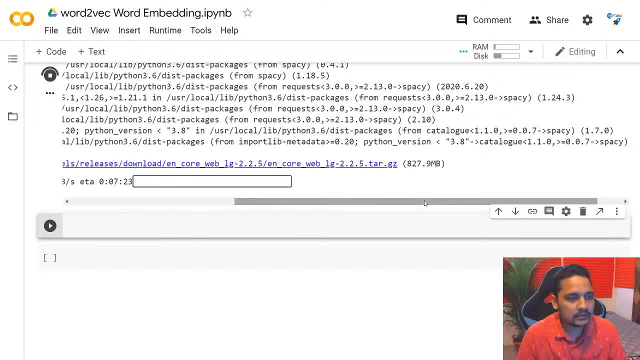 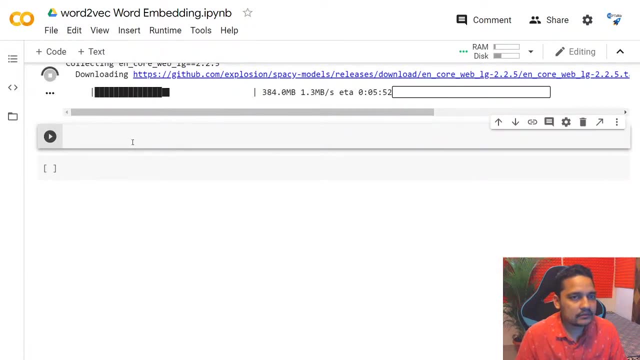 thank you so much. all right, so this large model is uh, around one gigabyte large model, so it takes it takes some time to install it on a google colab. once this installation is done, then i'll be showing you how you can let. let me fix it first. 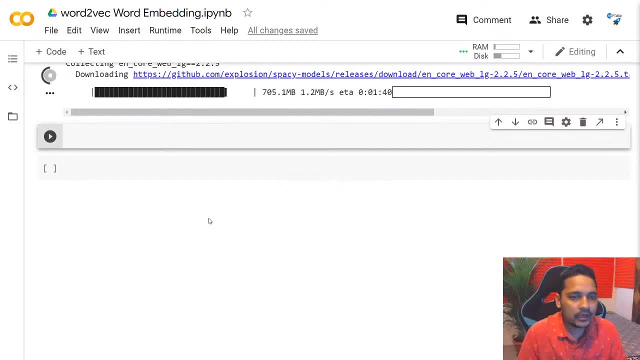 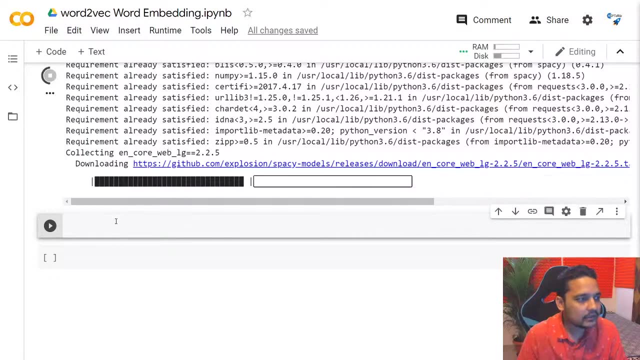 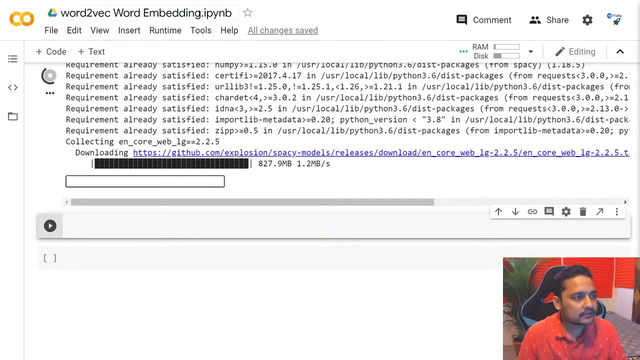 all right. so i'll be showing you how you can- um, you know the- read the csv file from the internet directly, and then how you can get started working with this word to vector word embeddings. so the moreover, you can also say that we are gonna do here. 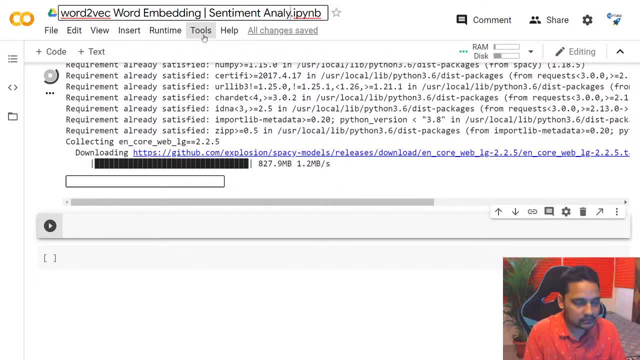 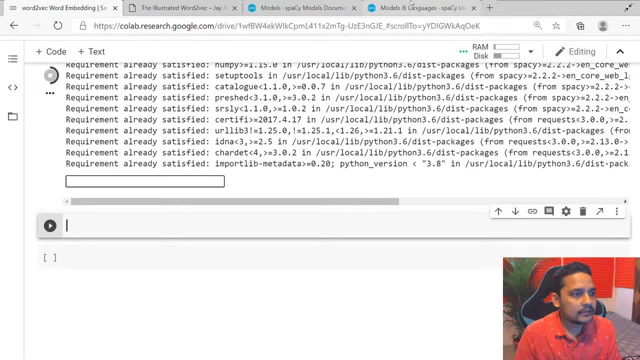 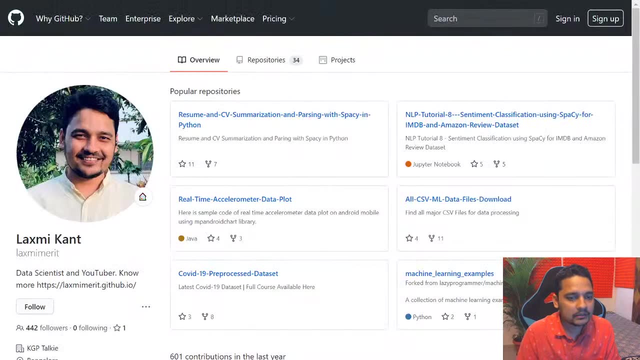 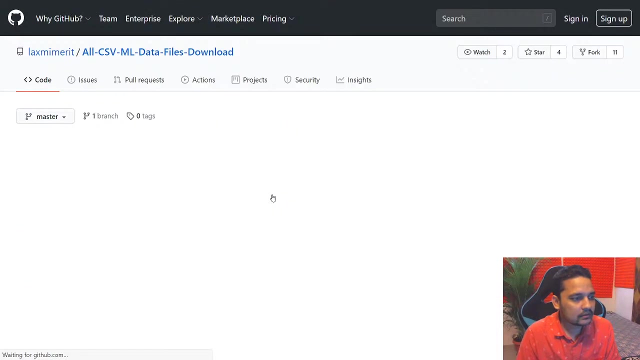 a sentiment analysis. all right, perfect. so to do that, we are going to go to the word embeddings and we are going to go to the word embeddings and we are going to download our data set. you have to come at my github repository and at that github repository i have- uh, i have there all csv, ml data files and in this we will be downloading here. let. 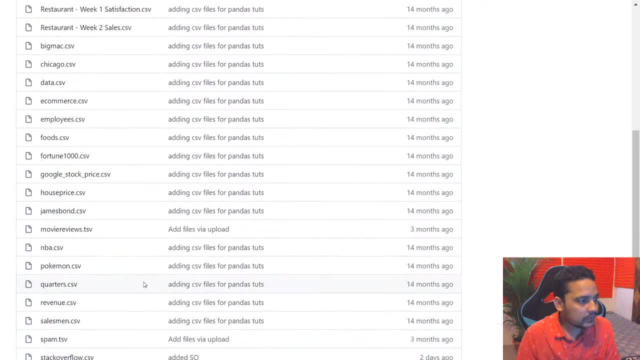 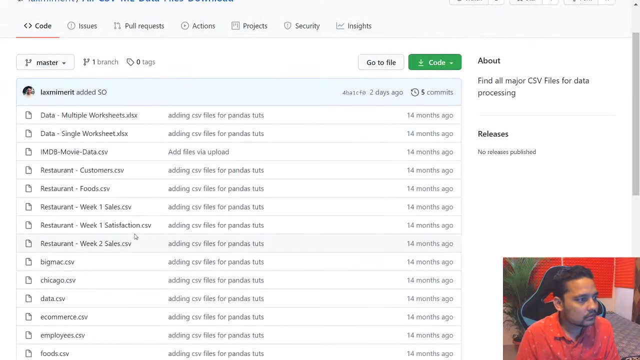 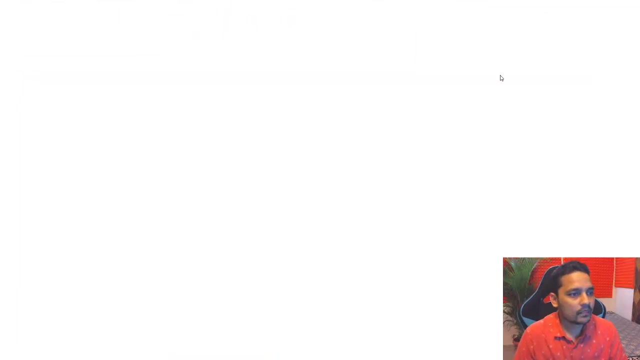 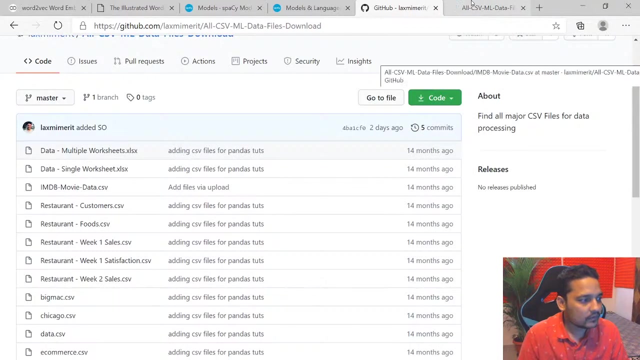 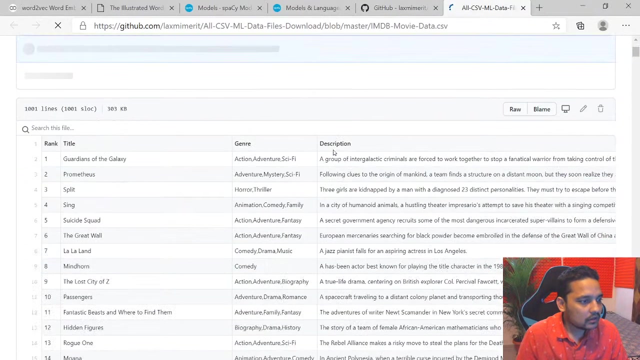 me get that one. we should have somewhere imdb movie database, i think this one, let me get this one first. so i think the internet is a little slow, so it's taking a little some time. otherwise you can open it here itself. not an issue, all right. so it says that it's a little slow, so it's taking a little some time. 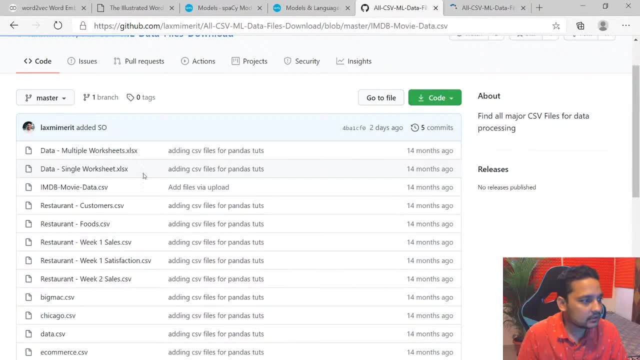 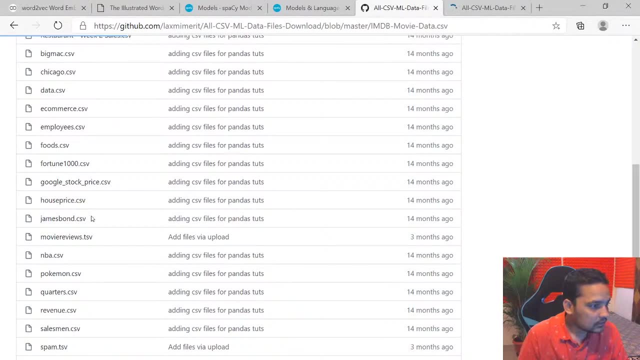 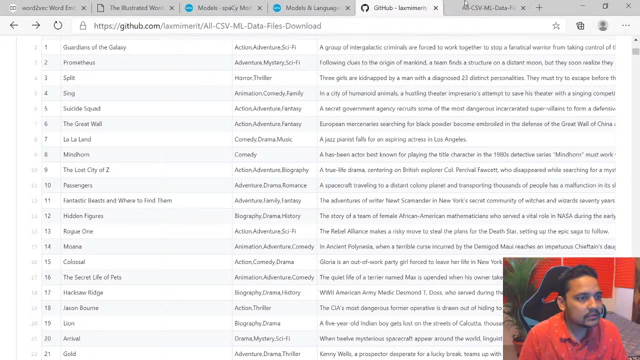 it has here a title. i think this one is jenner uh prediction. so we don't need that one for a jenner, we don't need. let me get the exact file. i think this tsv file, perhaps this could be. so we don't need this. um, this file is for movie jenner prediction that we can use in. 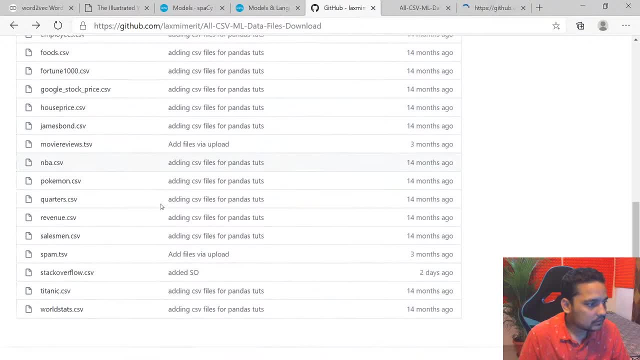 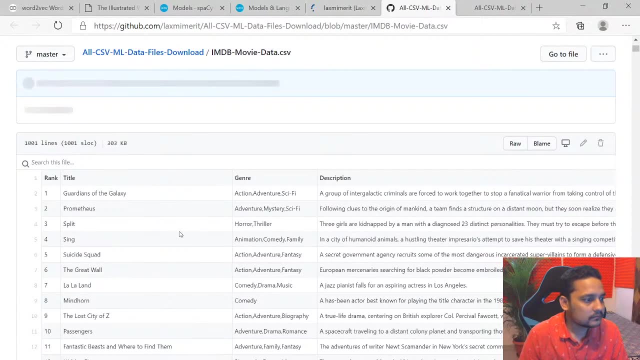 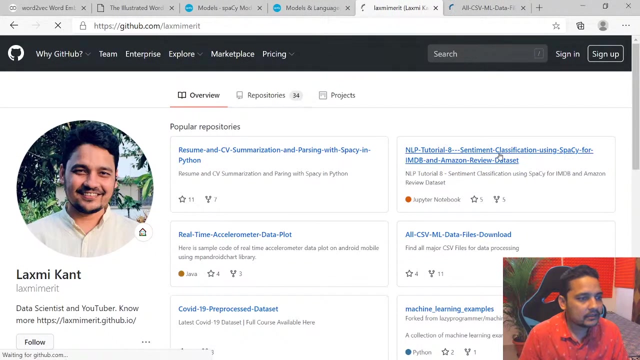 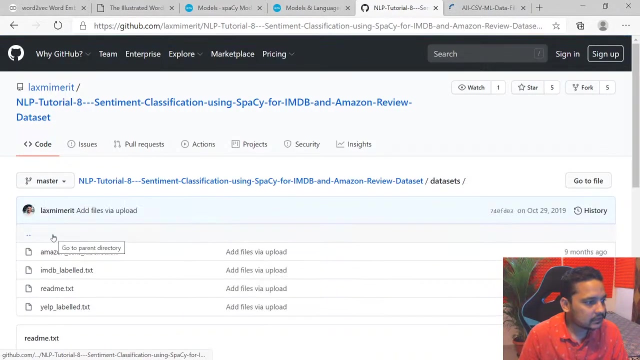 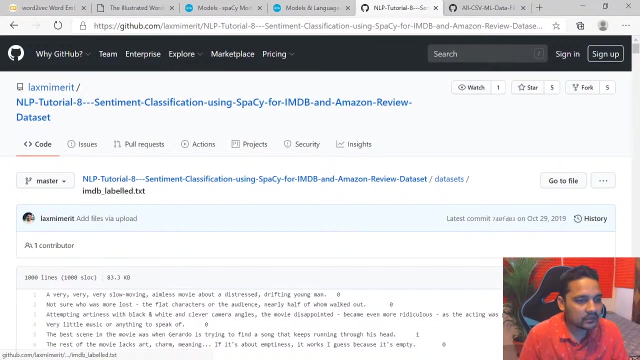 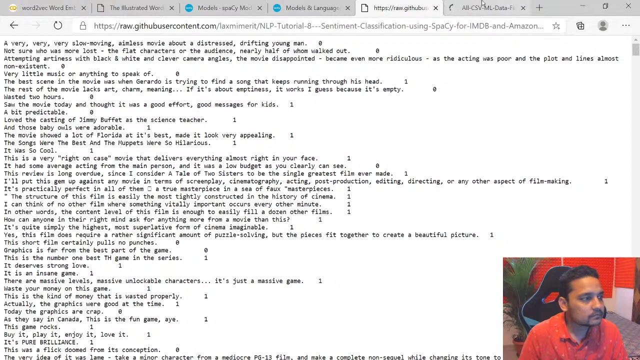 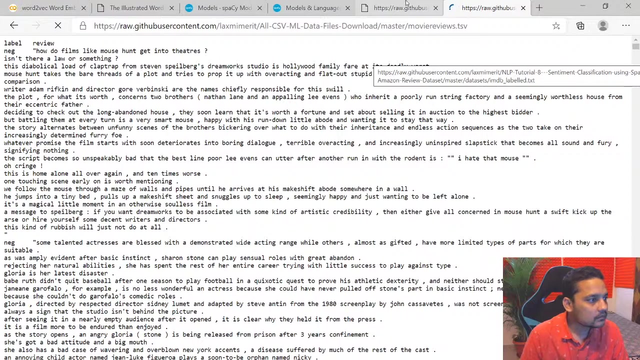 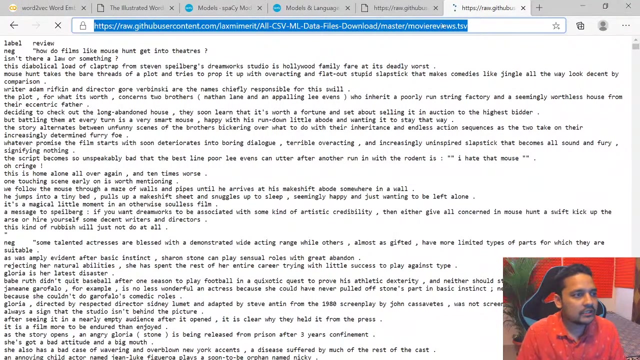 multi-label prediction. all right. otherwise, if it is uh not there, then we also have it here. all right. so in this we have inside this perhaps data set and there is imdb labeled underscore txt. then you can click on this raw. all right, all right. so there, you get here. movie reviewtsv say so, we got it. so this is uh. this file is. 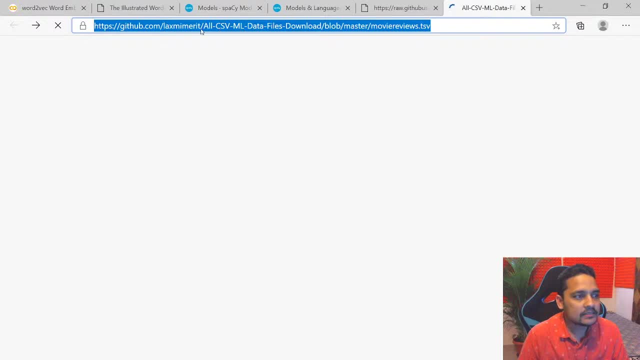 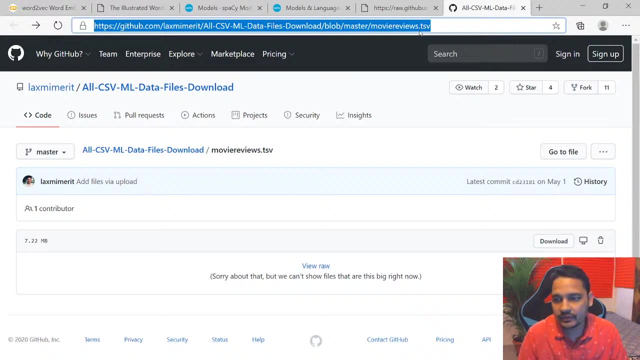 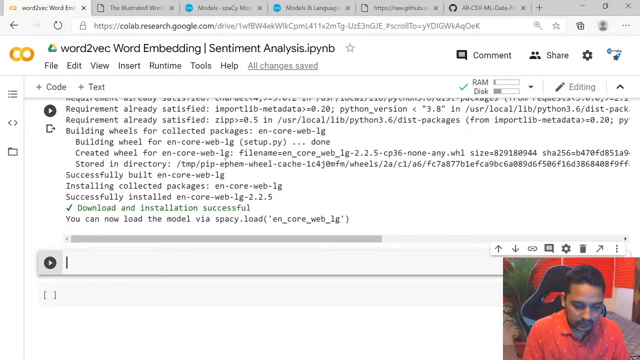 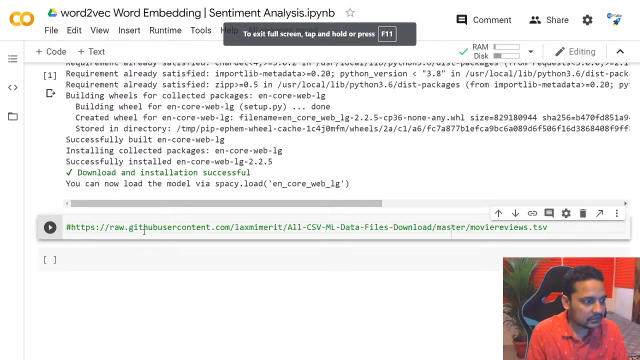 you can do again. this file is inside all csv, ml data files, download and movie reviews, dot, tsv. all right, so that is the file in which we are going to work. all right, perfect, okay, so we have downloaded our spacy model here, and then i'm gonna put this link here. 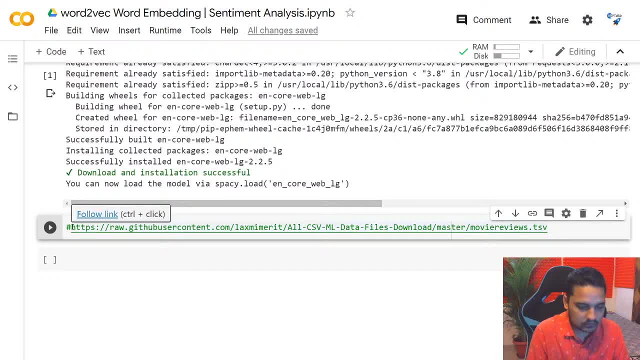 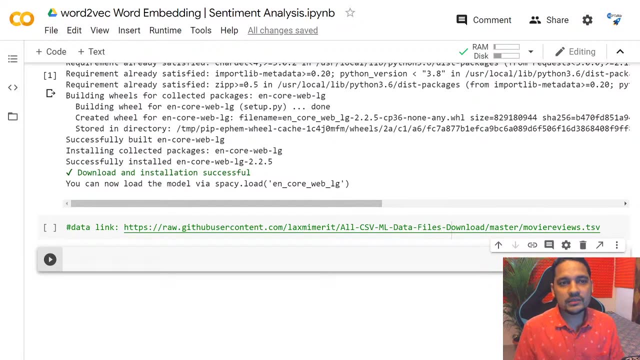 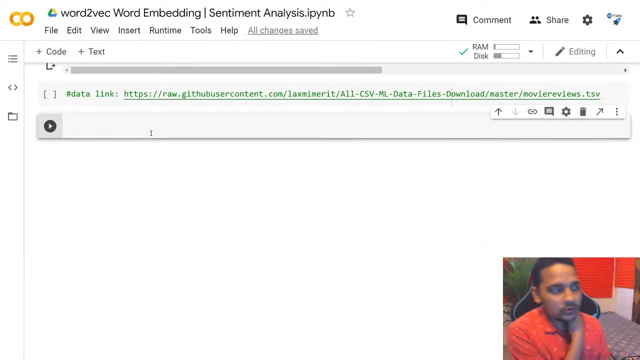 so that later i can use it here. this is data link. all right, super. now let's go ahead and import a spacy first and do some pre-processing with it. spacy so that we can get to use with a spacy. so the first pre-processing which i'm gonna. 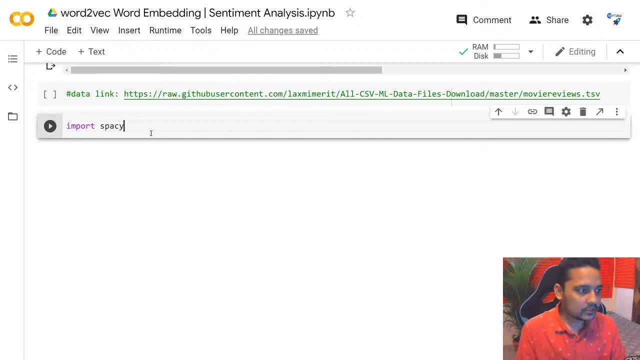 do here that import a spacy. so this is spacy. we'll import here a spacy object in your jupiter notebook. thereafter you can do here with the spacy dot load, and then you can give here this one. all right, i mean, this is spacy dot load, and then you can give here this one. all right, i mean this is. 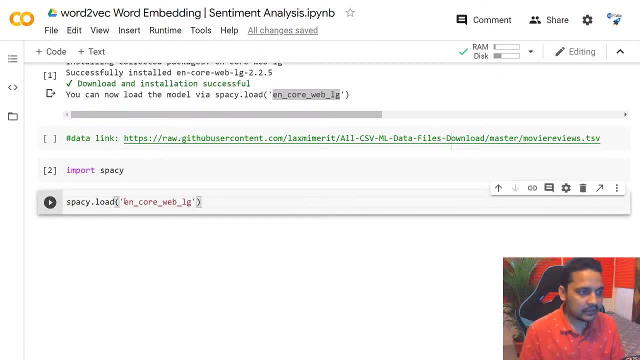 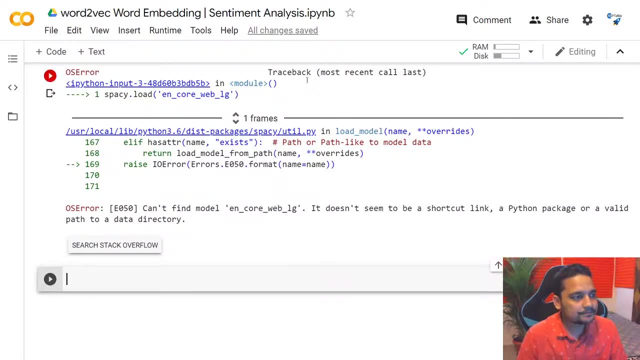 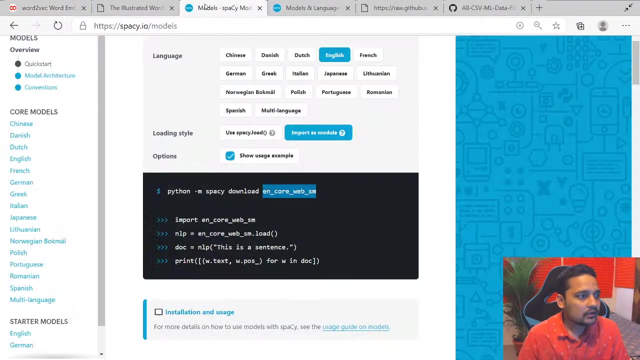 name of a spacy model which have a pre-trained vectors. so this will load a spacy. but sometimes what happen on google colab notebook? it do not find this as installed. all right, this model as installed in your google colab, so for that you have to read it in a different way and there it. 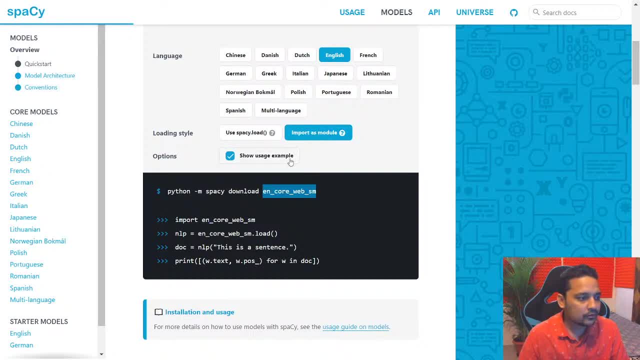 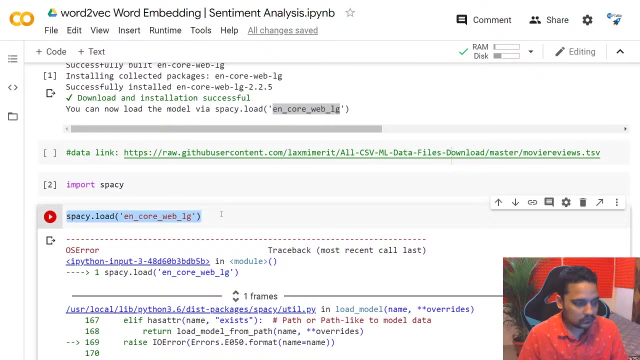 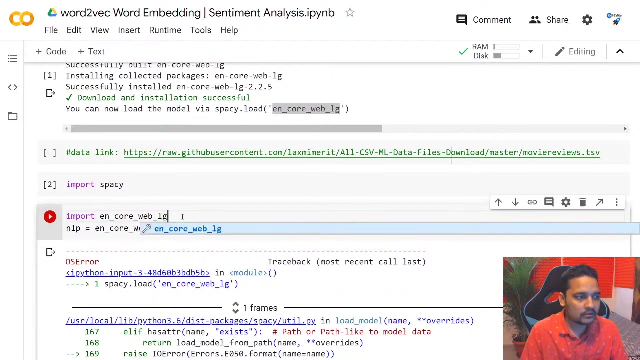 says that you can import it as a module and that module you can import it, something like this: then you import it and then finally you can load it. so let's go ahead and copy these two. so how it is doing here, it has imported this model, but we want here a large model. so 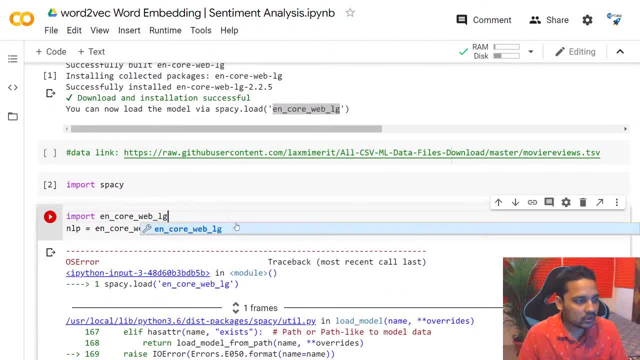 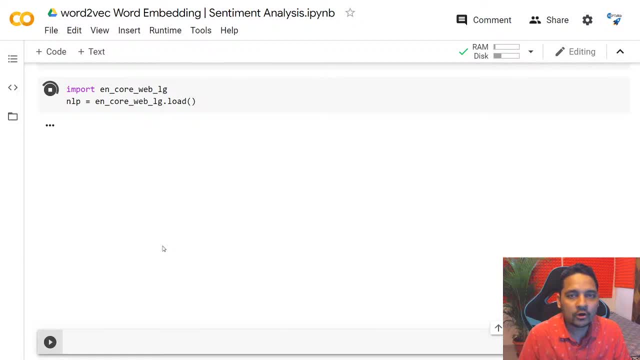 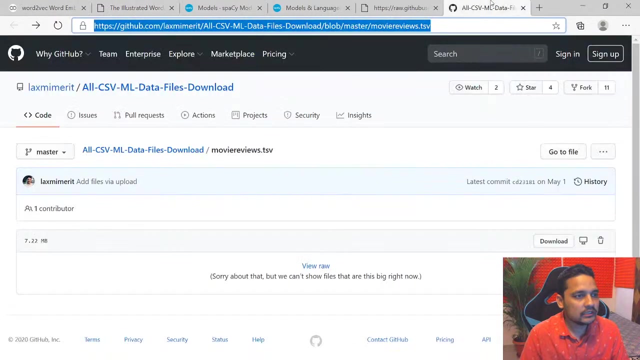 type there lg, that's the large model, and then here we have to also convert it lg. so with this we have got here our nlp object. now, once you got your nlp object, we can perform operations on the nlp object. but to understand how these nlp objects are working, one more thing i would like to show you here. like, let's say, 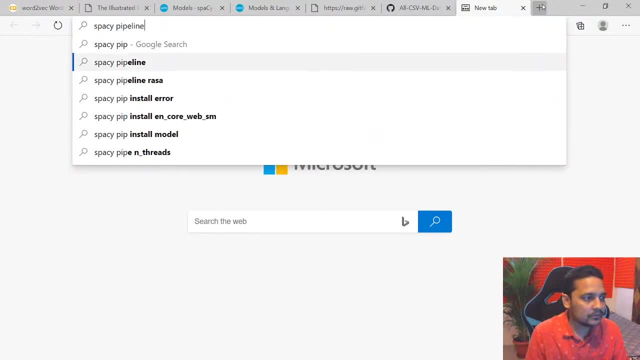 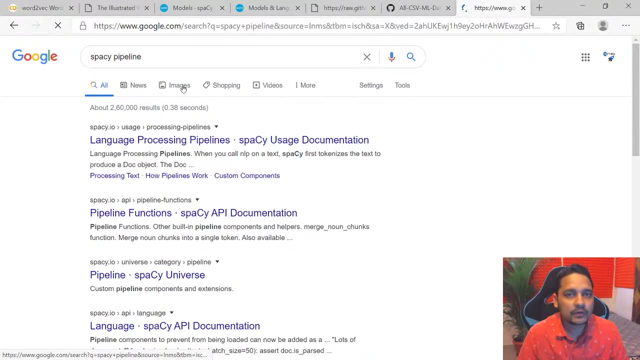 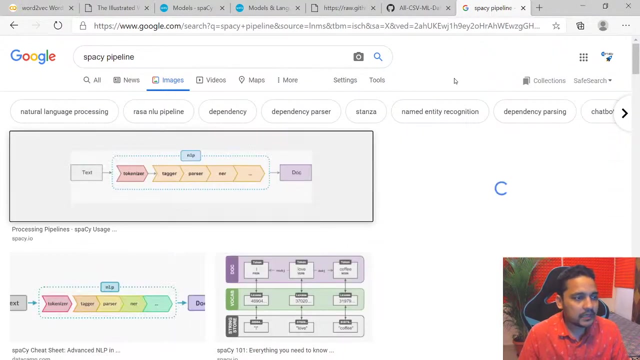 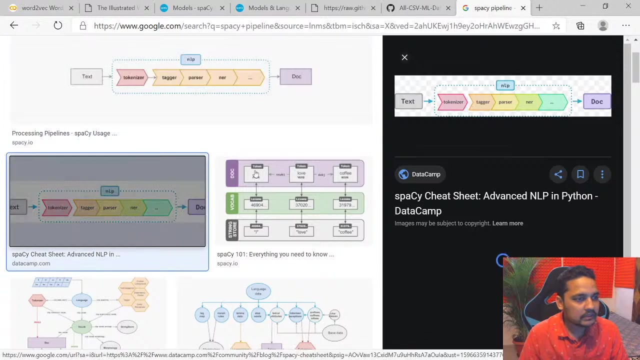 a spacy pipeline, all right. so if you search here a spacy pipeline, then you will get to know that how these spacy pipelines are working. let me show you here an image. all right, so this is a spacy pipeline image in this. if you, you should be able to see this one. otherwise, let me make it a little larger. 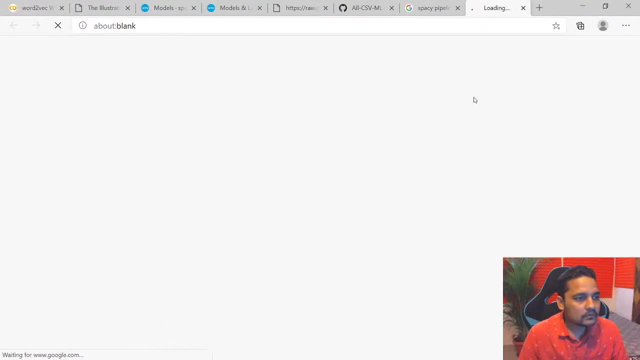 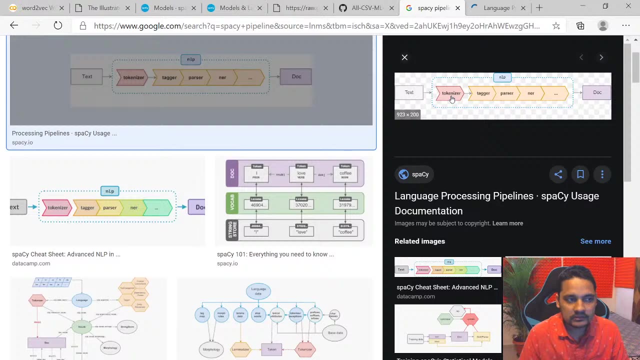 all right. so there, in this model, we have a text data, thereafter we have a text data, and then we have a text data, and then we have a text data. text data is being tokenized and then we have here nlp pipelines, and these are the nlp pipelines. 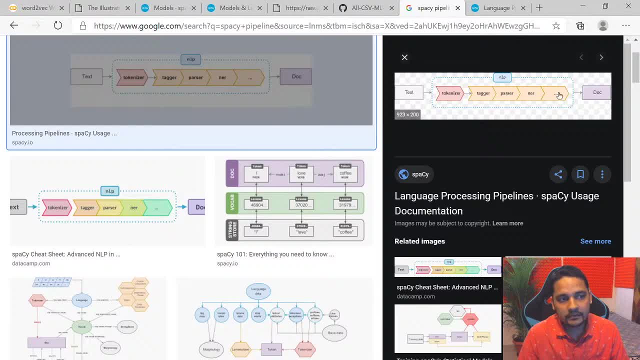 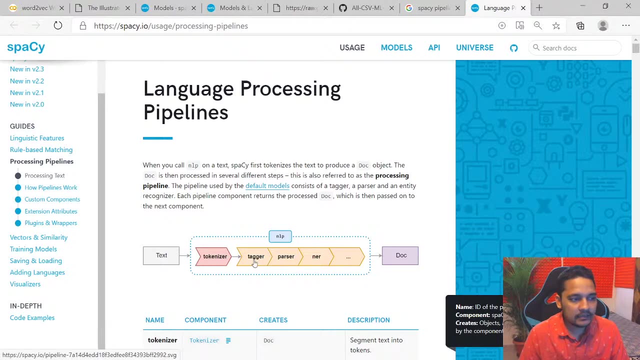 which are optional, but by default. these pipelines are included, like tagging, parsing and ner, and this is compulsory and this one is mandatory. tokenization is always mandatory, and only these pipelining, like tagging, parsing and ner. these are optional. so whenever you are doing tokenization with a spacy, then in any cases, in fact in all the cases, 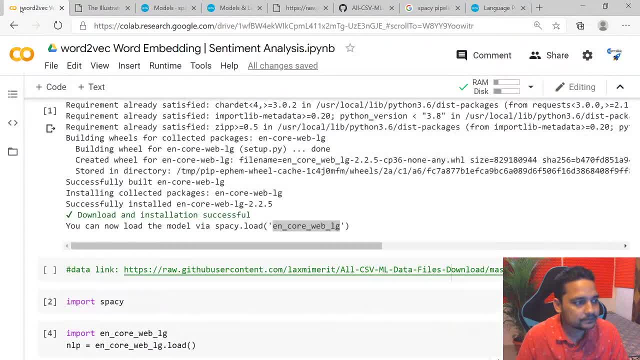 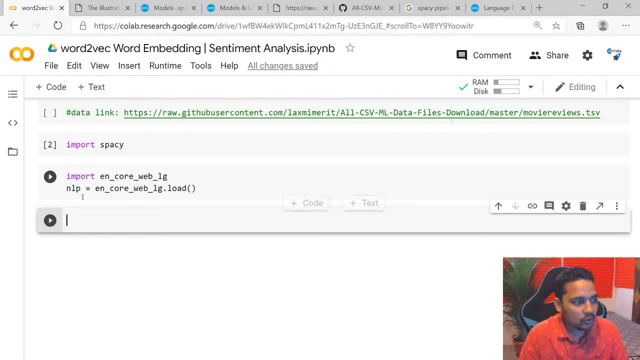 the tokenization will be always performed. so whenever you do like, nlp is equal to the en core and web lgload. thereafter, whenever you pass here any text data, then then that tokenization is always performed. all right, so let's go ahead and do it like this. one x is equal to, let's say, i want to do like a. 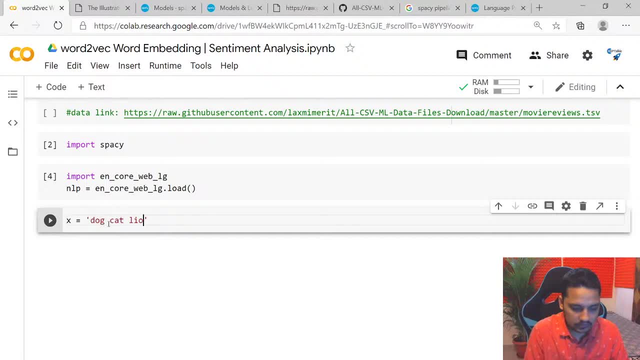 dog, cat and lion, and then i'm gonna put it here some wrong spelling. thereafter i'm gonna create here a doc object. so this doc object says that doc is equal to nlp and then x. so with this we have got here a doc object, and then we have got a document. and then we have got a document, and then 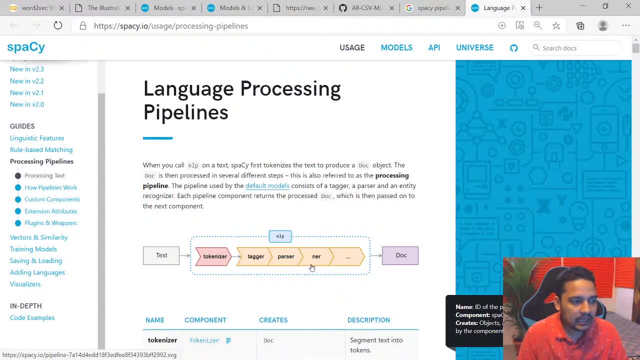 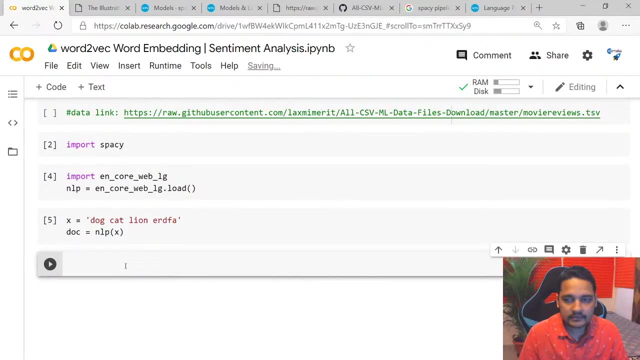 this doc object is having tokenization, tagging, parsing, ner, all those things are by default performed on our text data and those information and results are stored inside a doc. all right, then what's happening here? if you do like this doc now, the first of all, we are going. 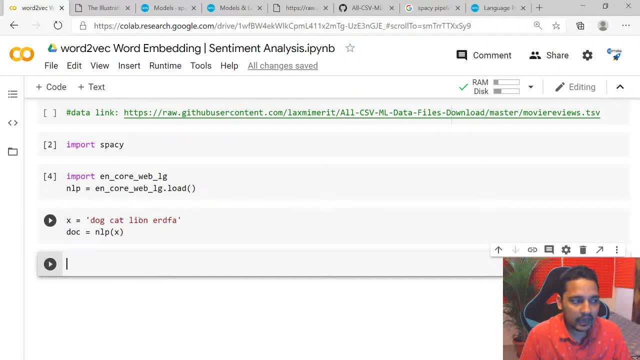 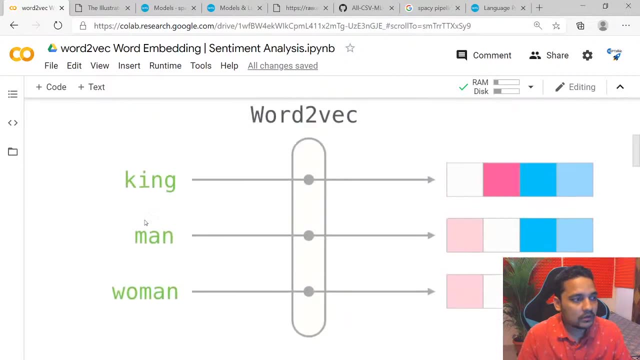 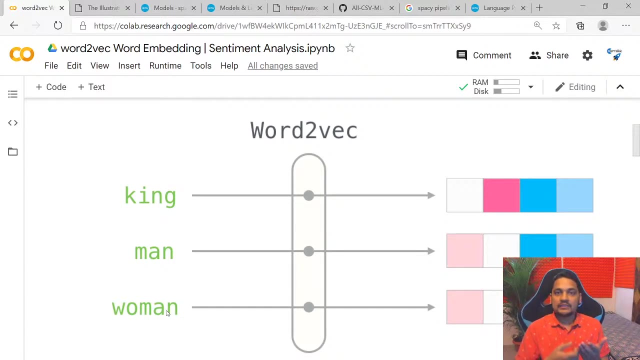 to see that how much these dog, cat and lion are similar to each other. if you remember, previously i talked about how these words are similar and if they have high similarity- i mean the similarity coefficients are high- then they will be placed placed in a same coordinate, or 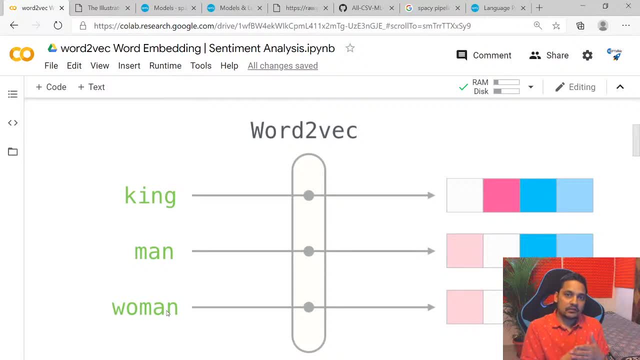 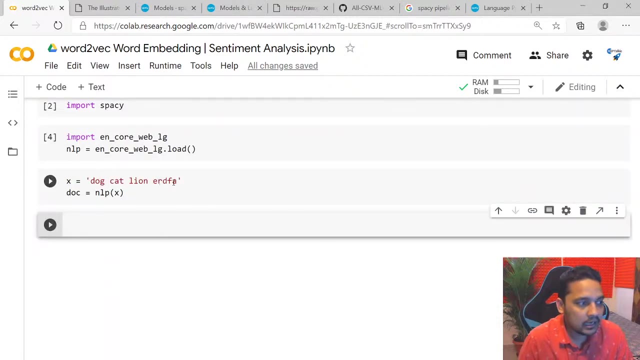 in a same dimension, or you can say a nearby dimension. that's mean if they are in a nearby dimension, that means the similarity is high and the same thing. we are going to test it here. if we write their dog, cat, lion, all right, and then we will see how much similar they are to each. 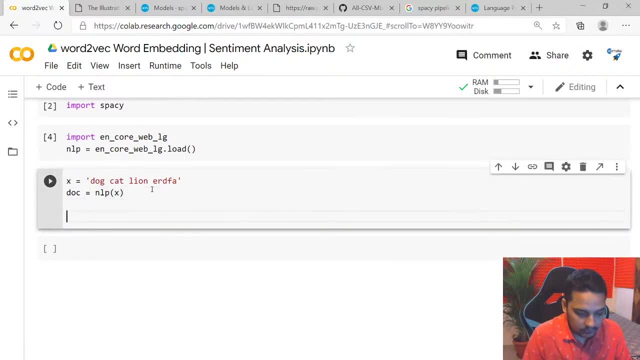 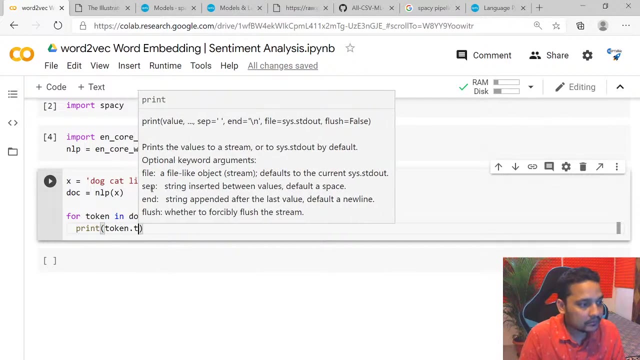 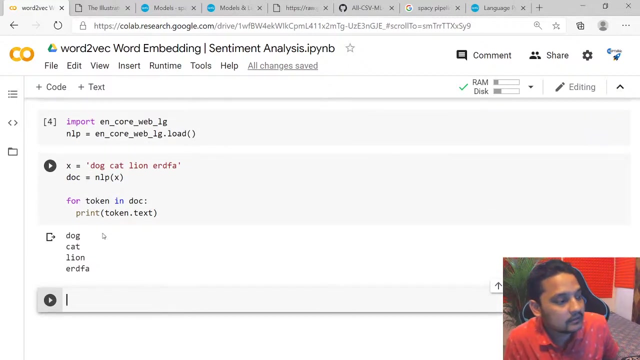 other. then i'm gonna do here for token for token in doc. thereafter i'm gonna print it here, the similarity and the similarity how you can get it with the tokentxt data. you will get here the token, get here the tokenized text data, like a dog, cat and this lion, and that up this. 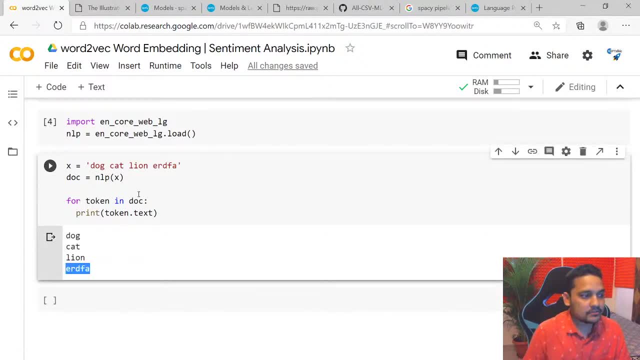 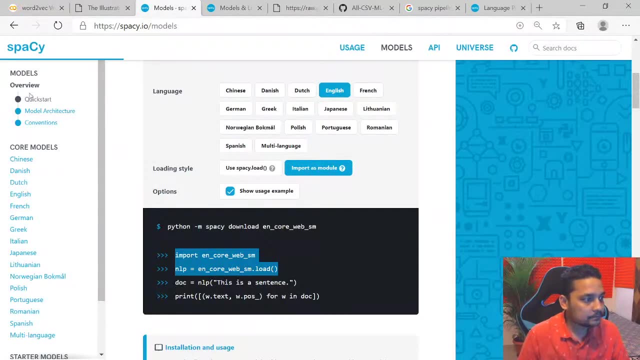 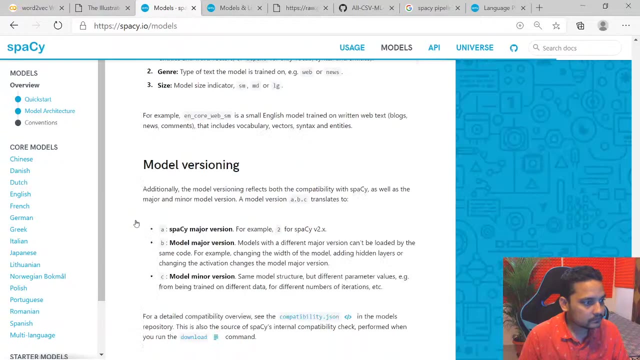 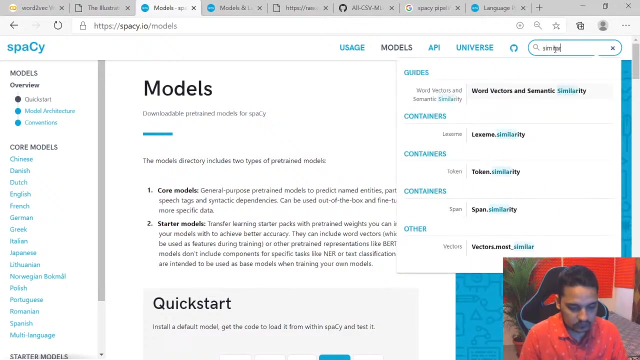 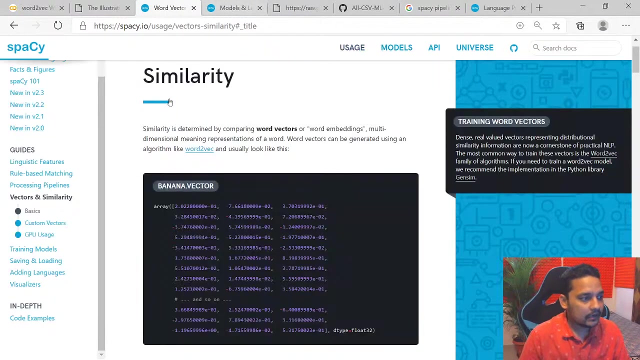 one, all right. thereafter, once you have this one, then we can test the similarity. and to test the similarity, let me show you here in the quick start guide you will be having you should be having here. let me see it here, all right, it's not there, if you. so there is very good guide available on a similarity on this. 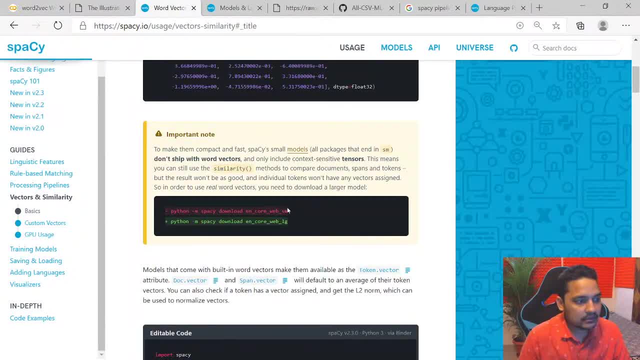 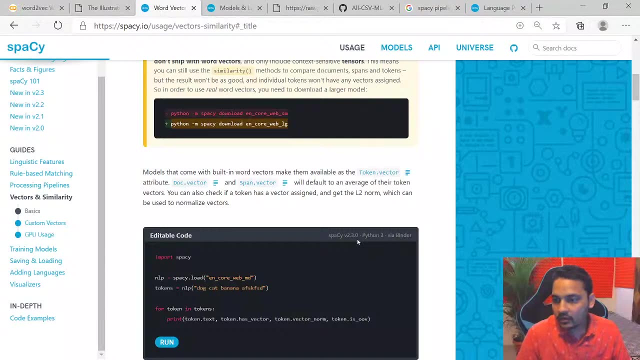 especially so. the similarity says that we can't work with a small model, but we need here large model. that is what we have already done in our notebook thereafter. all right, so we seeing is asking about make a video on excel, net and robot. yeah, definitely so I. 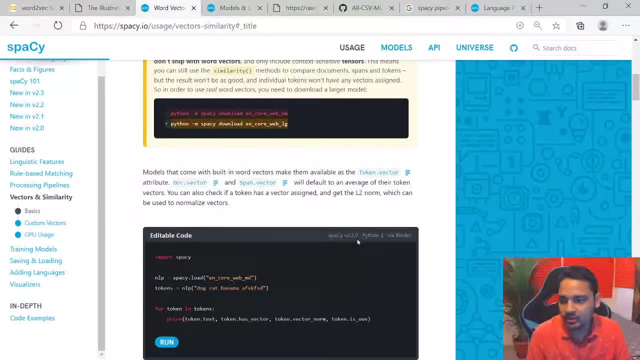 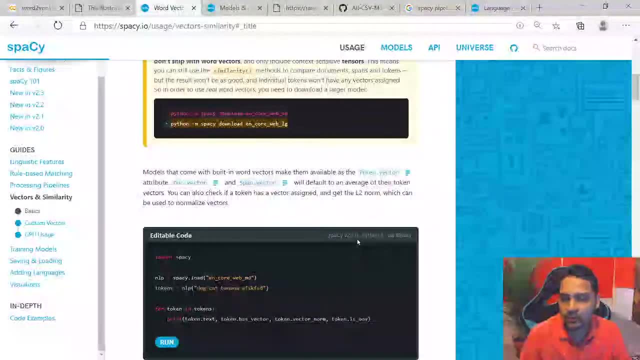 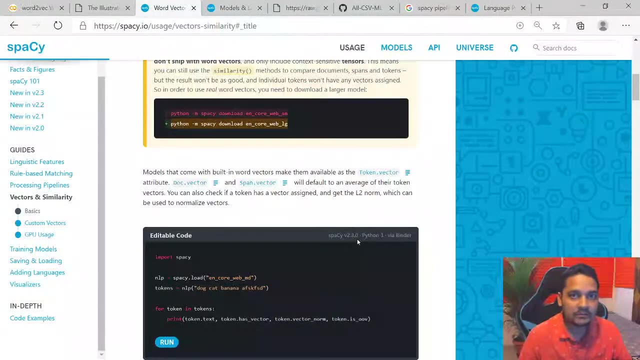 have a plan to make on make videos on excel net and robot. definitely I'll make. but if you are interested to you know about like but and distilburt and fast text model of those models are pretty much advanced NLP model so I have already a made a few videos on those. so 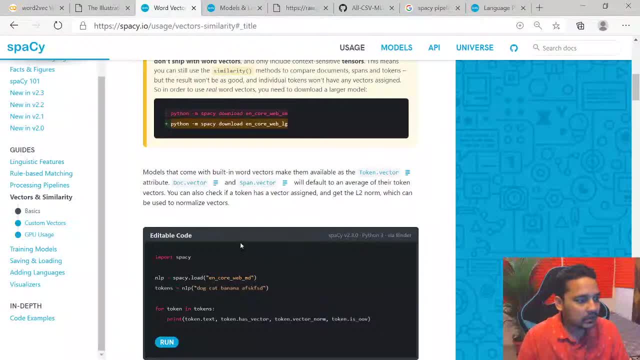 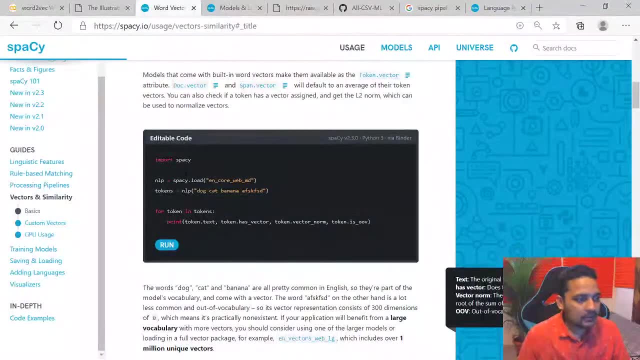 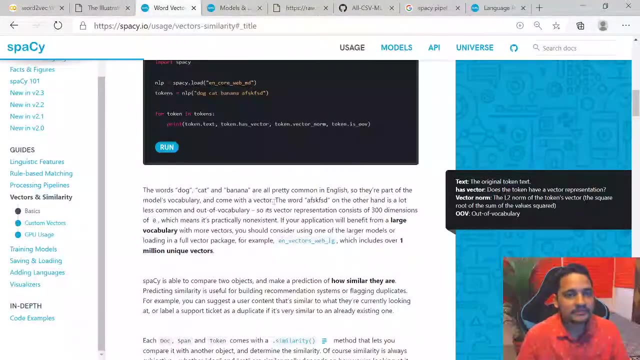 you can see those on our NLP NLP playlist. all right, so we are talking about here how we can find out how much you know correlated they are to each other. alright, that's mean the similarity map matrix. so there, you can follow this guide. otherwise, let me also show you how. 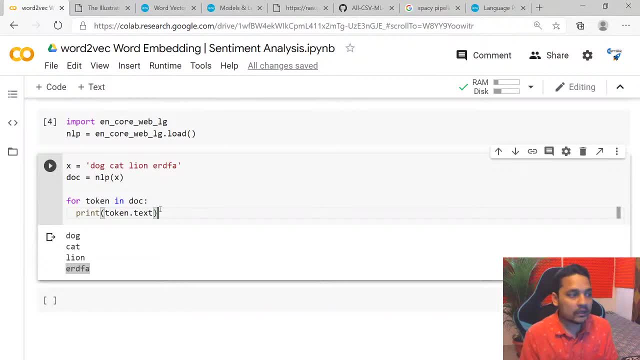 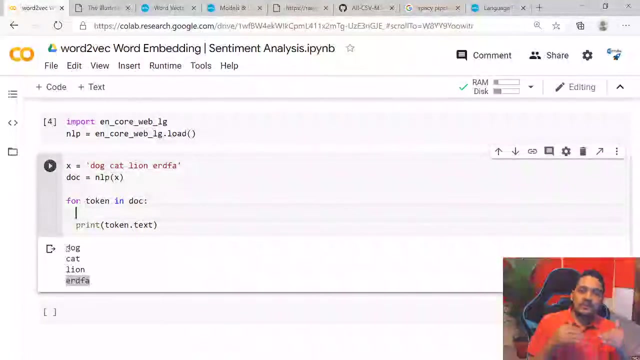 you can find out those similarity between one, between one token to another token. all right, so there we have token. now we have got these four tokens. now we have to make here a four by four matrix so that we can represent similarity matrix between one token to another token. and for that one we have to. 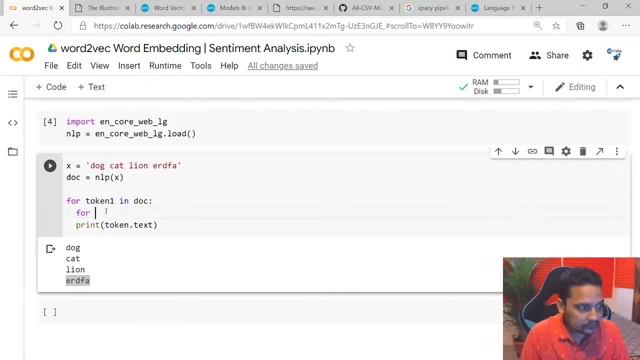 iterate it two time. so thereafter for token 2 in DOK. all right, superb then what you have here: token 1 and token 2. there we have token wanted, token 1, token 2, token 1, token 2 and token 2, token 1, token 2, token 1, token 2, token 2, token one, token and token 1 and token 2. there we have token one text. 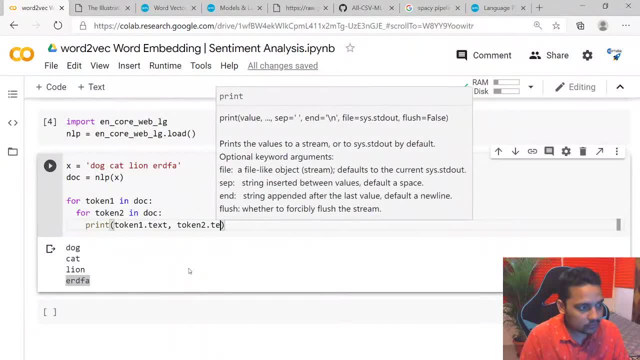 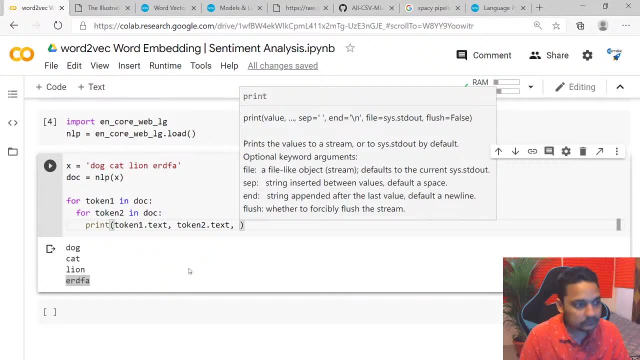 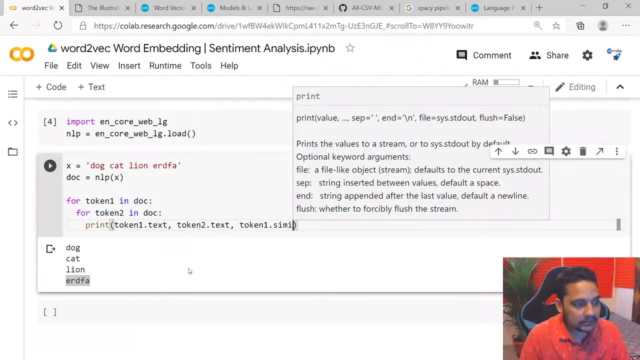 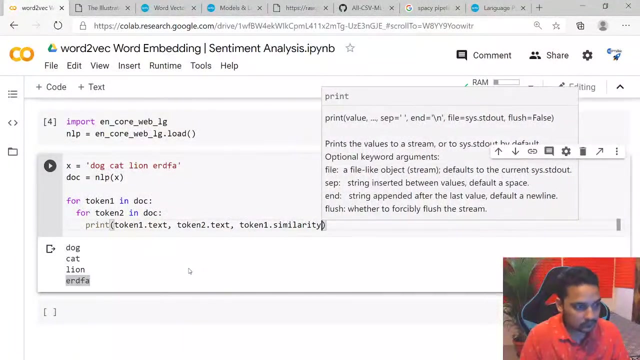 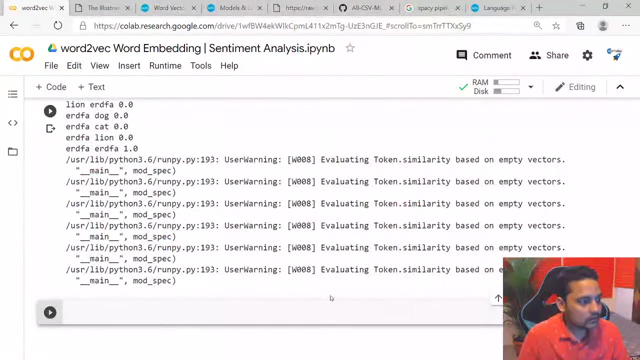 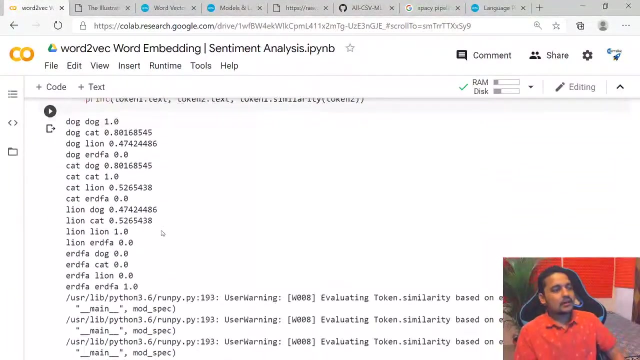 and then I'm gonna say here, token two, dot text and then I'm gonna type their NLP. actually I need to get here this token one, similarity with the token two. all right, so you can type their similarity with the token two. all right, so what it says? that here you have got a similarity matrix, but at the 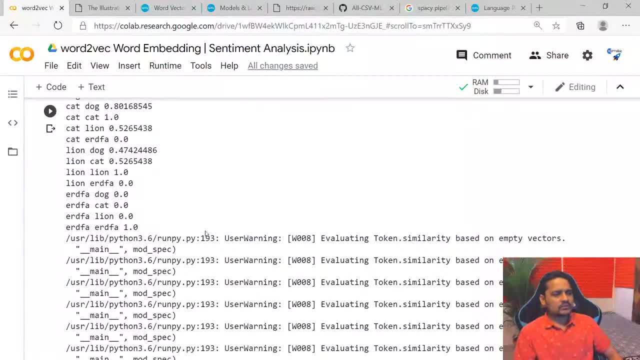 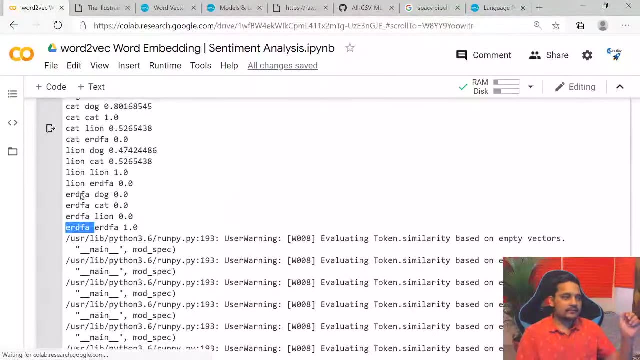 same time you have also got here error. so it's not the error, but it's kind of a warning. you might ask that why is it not working? why we get this warning? we got this warning because especially do not have any word to vector representation for these particular words. I mean for this: 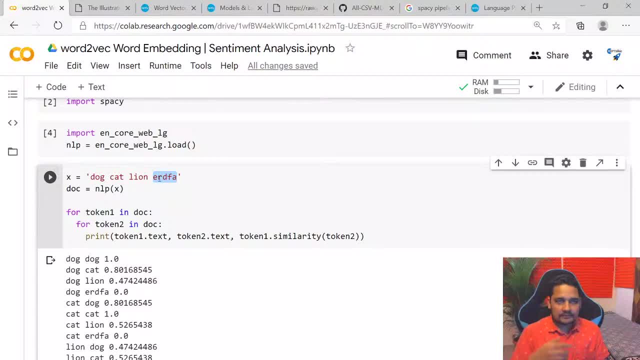 token. so that is why I had, you know, placed that misspelled word there and I did that intentionally so that you can get to know that when you do not have a word in your word to vector representation, then Spacey will return there a zero vector, and if you try to get the 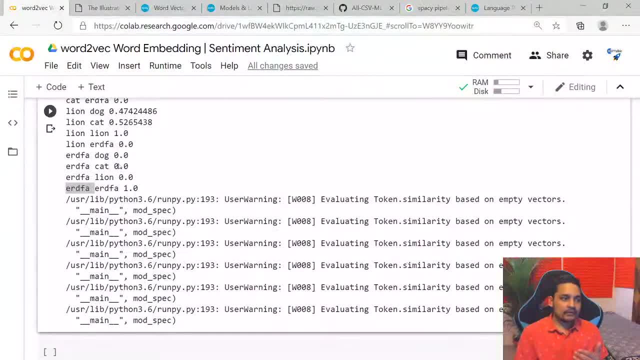 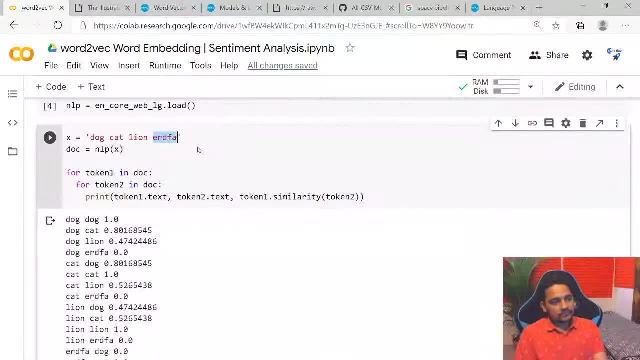 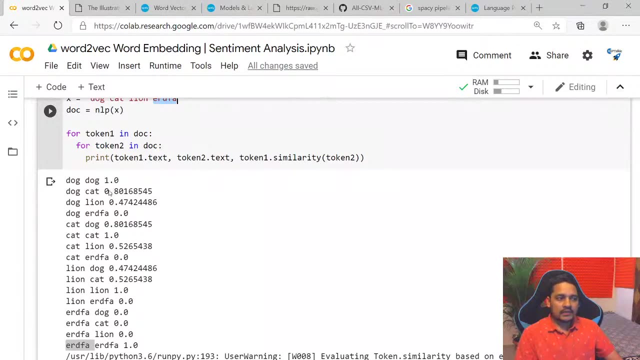 similarity. with the zero vector you will always get there a zero similarity, all right, but of course word towards similarity will be always one, all right. and apart from that, if you notice there a dog to dog is of course one, but dog and cat similarity are 0.8. it's pretty much high and it should be, because dog 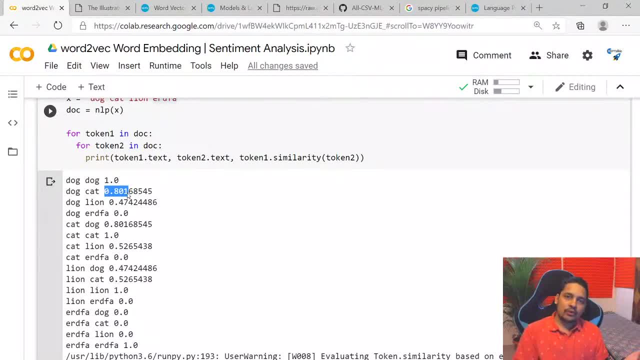 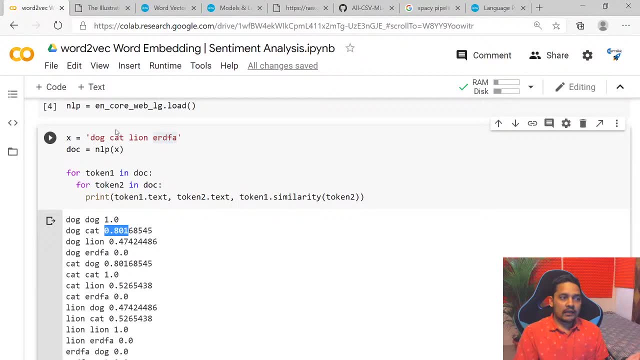 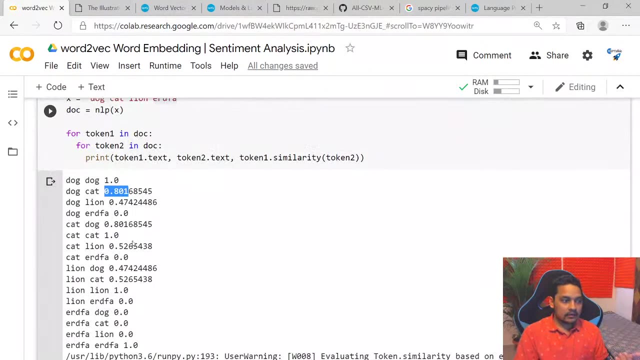 and cat are similar in the sense that if you get to know the word a, then that's that if we talk about the animals there, we have a lion. so if we talk about this dog and lion similarity, then we will get high similarity for dog and cat instead of dog and lion and at the 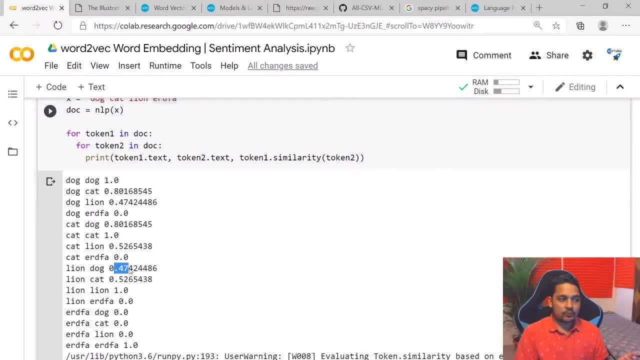 same time, if you see this lion and dog similarity- that is 0.47- but at the same time, if you see this cat and lion similarity, then you have a high similarity than this dog and lion and if you think about this, you will get to know that. 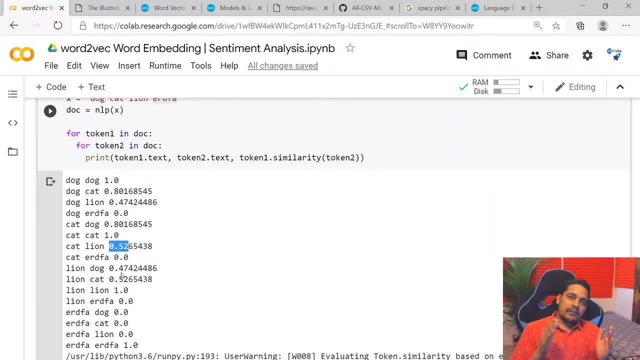 if we, if we are given only two option that we have to find out best similar match in between dog and lion, cat and lion, then definitely you will select their cat and lion all right, like cat, tiger and lion. so they kind of falls in a same category than dog and cat, because those are completely different. 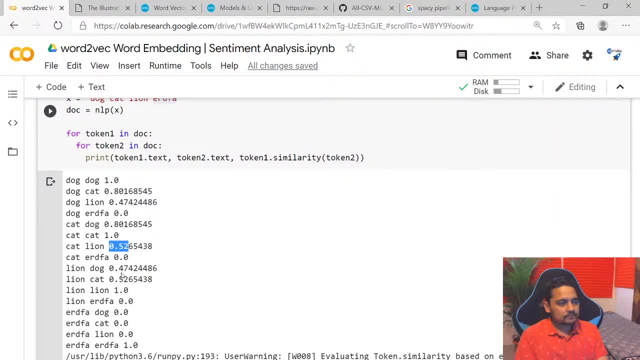 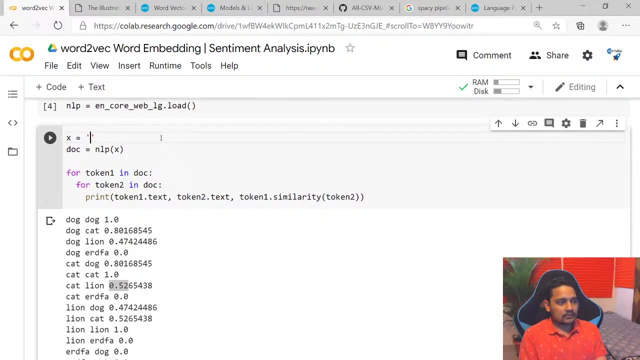 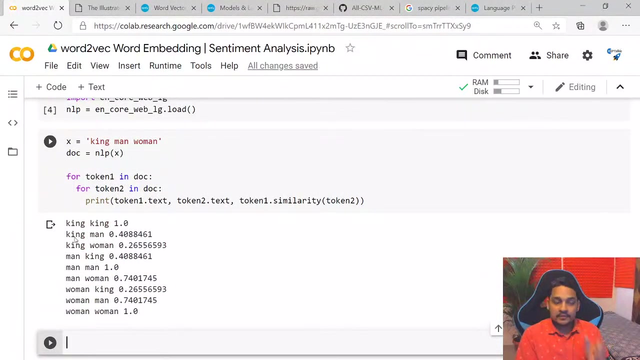 to two type of the different animals. and similarly, if you put here: let me remove this one, apart from that one, let's go ahead and put here this king man and this one omen. and now, if you try to see here similarity, then you will. you will get here a similarity between this king and man instead of 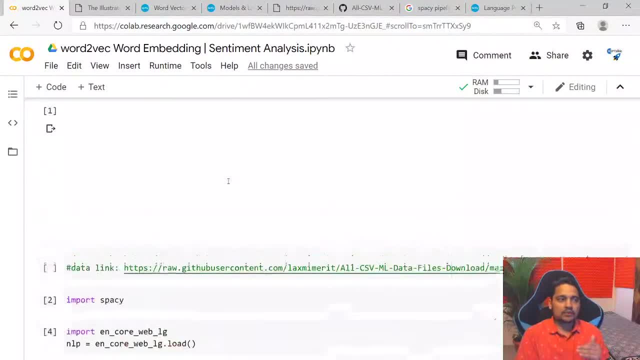 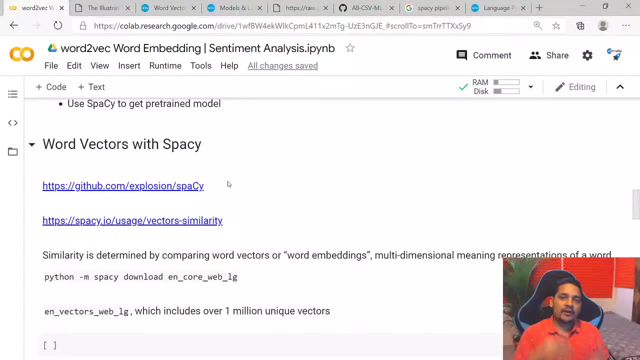 this king and omen. all right, that is what i was talking about here. so this word two vector representation is, you know, very beautiful. it try to find out the meaning of those words and what are actually what they are representing and how much they are similar with the other words. 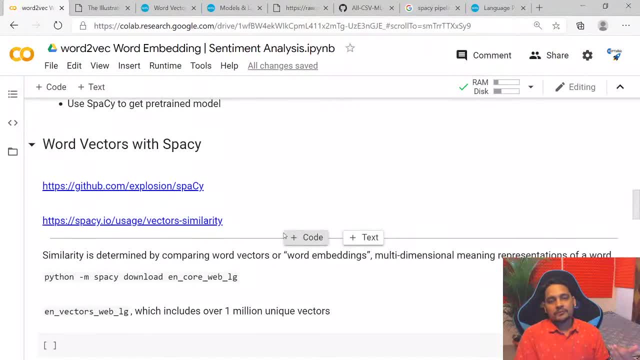 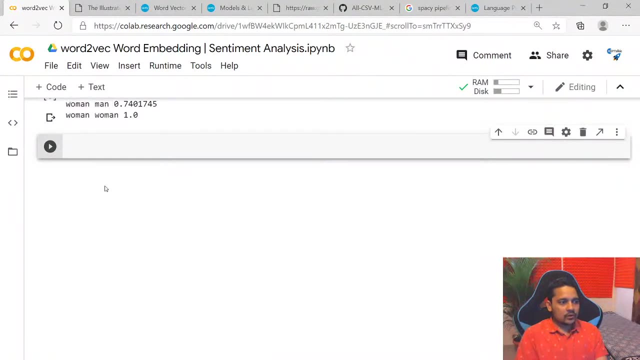 so based on that one, we can also find out the sentiment pretty much. you know accuracy with the pretty much good accuracy. all right, so we are done with this one. let's go ahead and build a model. all right, so we are going to now build a model. but before we build a model, few things we have to do. 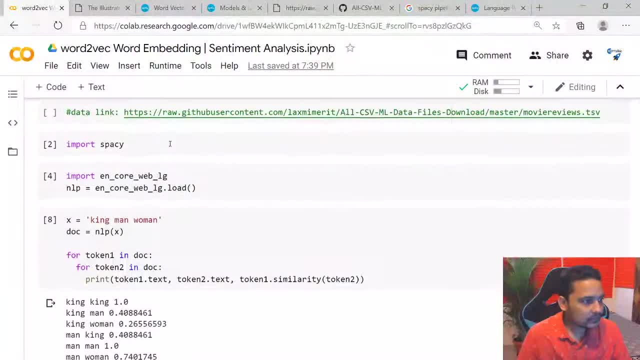 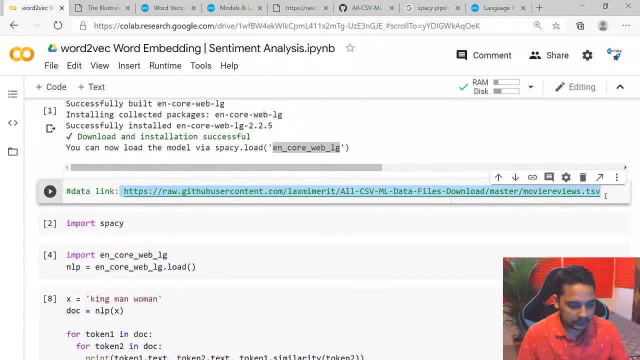 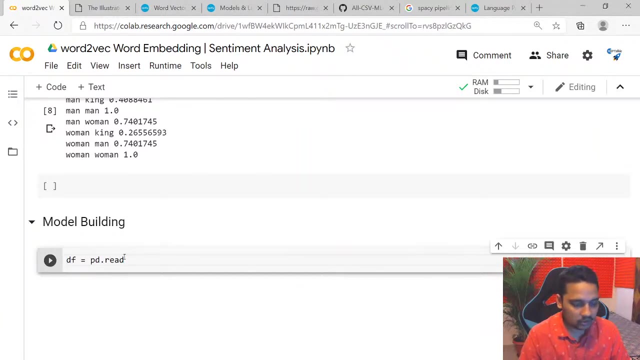 first of all, if you notice, we have not read our data set, so we have to take, we have to read our data set. so the link of the data set is this one and we are going to read this data set directly from the internet. so the pdread. 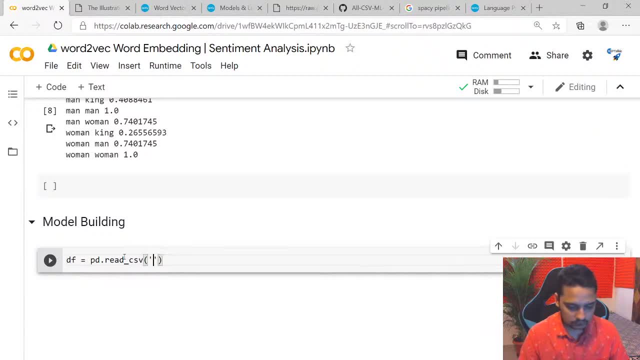 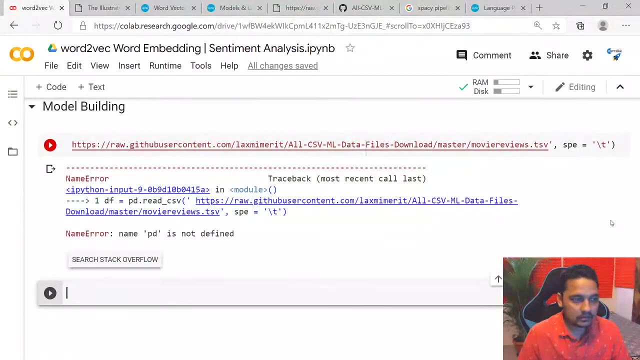 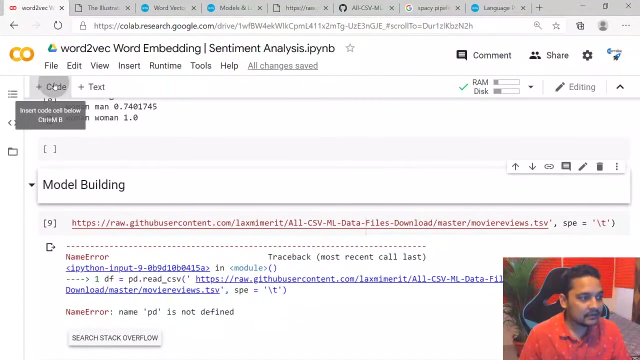 pdread underscore csv. but if you notice that this is tab separated value, so you have to define here separator, which is a tab separator, all right, and it still says that. okay, so the pd is not defined. we have not defined any. the codes. are it sorry? by default i had added here. 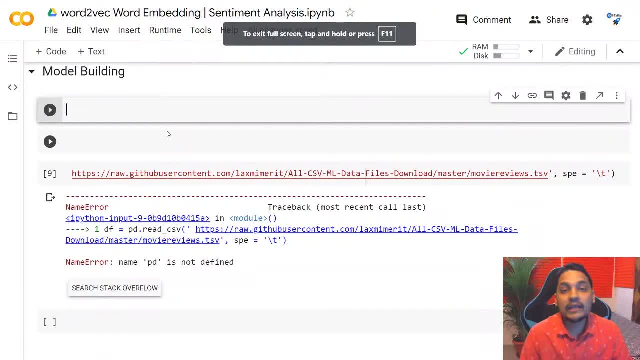 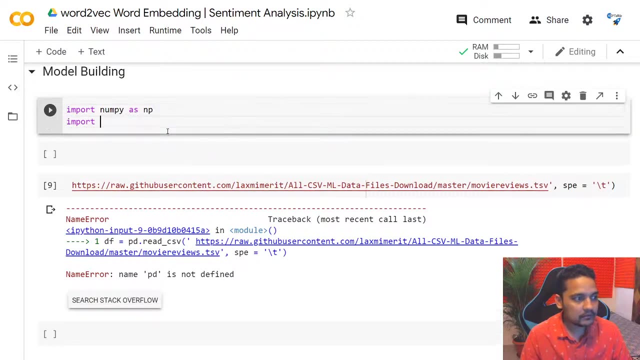 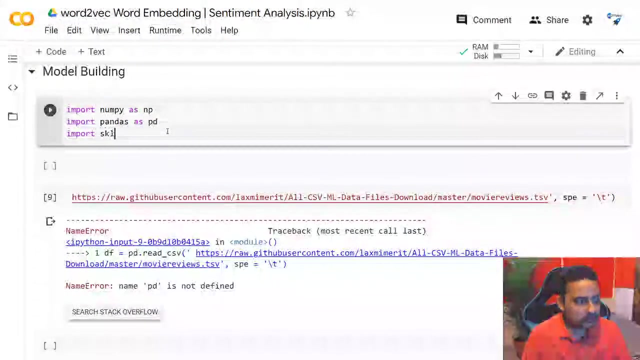 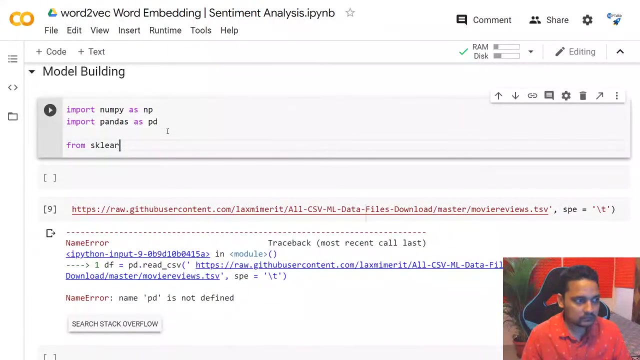 all right. so the first of all we have to import our numpy, pandas and other necessary python packages in our notebook. so we are going to do here: import numpy as np, import pandas as pd. then we are going to import here- sorry, from a scalar dot your model. 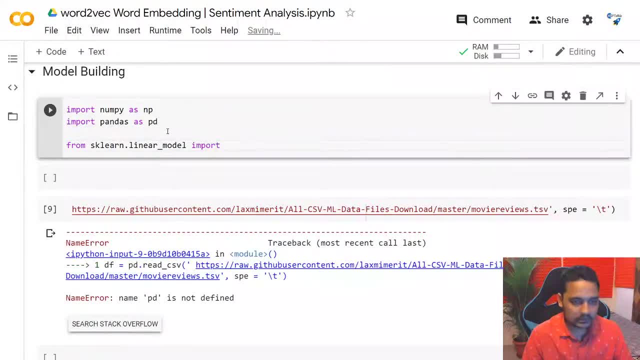 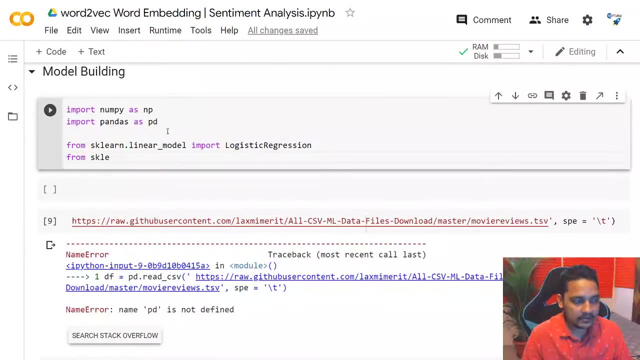 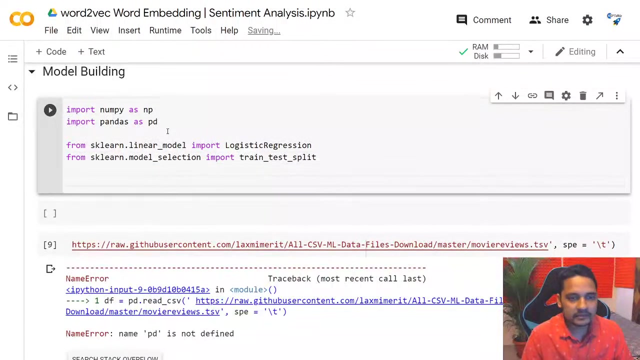 thereafter, i'm gonna import here a logistic regression, so we'll be using here a logistic regression with this word to vector. thereafter we have here a from a scalar dot model: selection: import: train test is split, all right, perfect. thereafter we are also gonna get here a classification report from a. 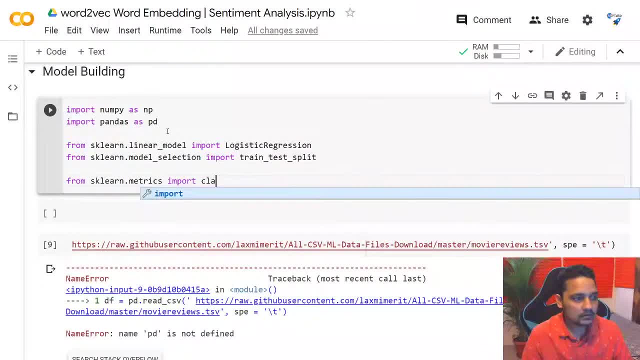 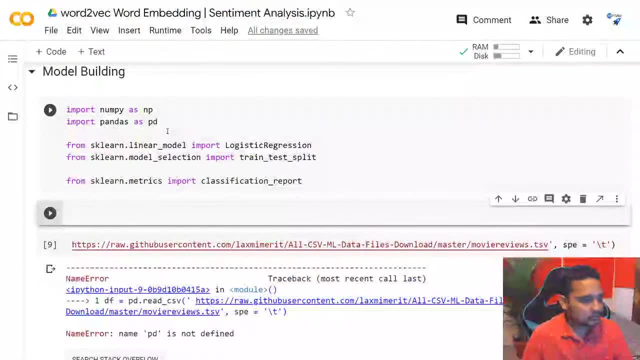 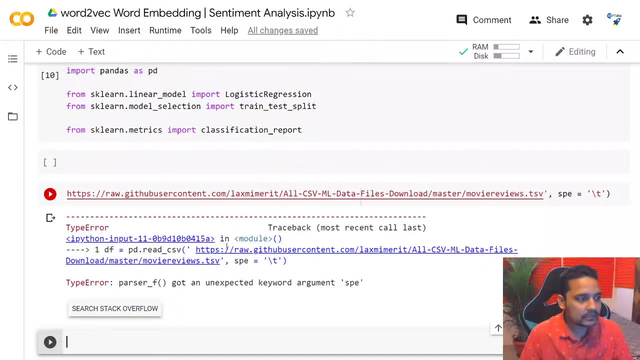 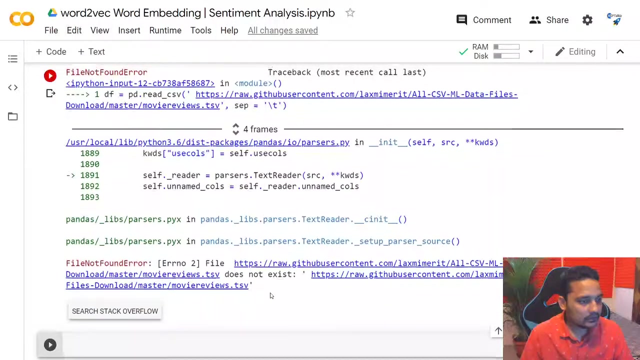 scalar dot matrix import classification report. all right, perfect, super. so we have imported here necessary python packages. now let's go ahead and read our data set from the internet directly. it says that, okay, this separator should be a sep, sip. all right. it says that this file does not. 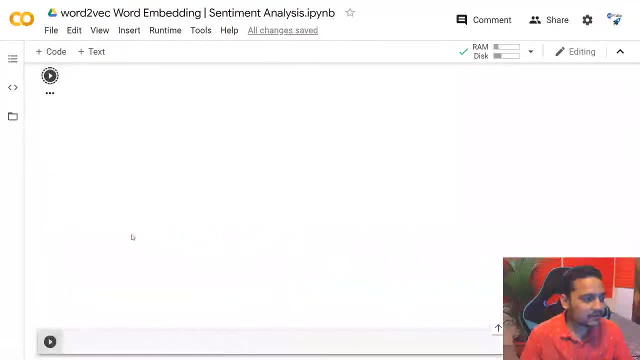 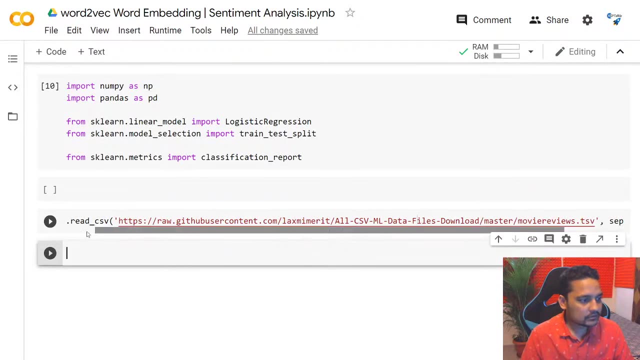 all right, i think they have. there is a space, all right, so we have to remove that space. all right, so we have got it now. let's see, we have got it in data frame. that is df. let us called it 다니. so there, it is okay, this sep sip. 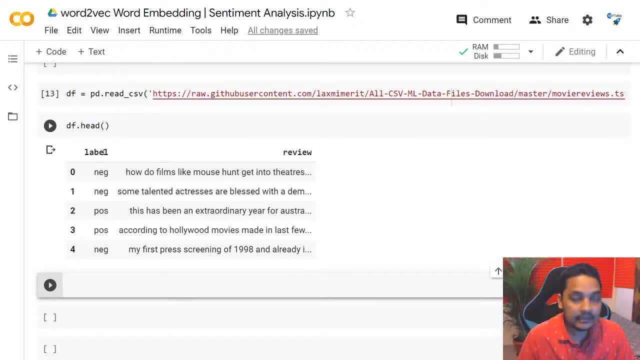 already pipe, do not go away. got it, can get it with the bfhead, all right. so in this data frame we are having here a label, so this label is a target breach able, sorry, and label is a target variable and we have the review when we have these double line associated to one folder library only to frame: Всем k могу RSVP parents for outstanding among our people and we have the review, so that's. 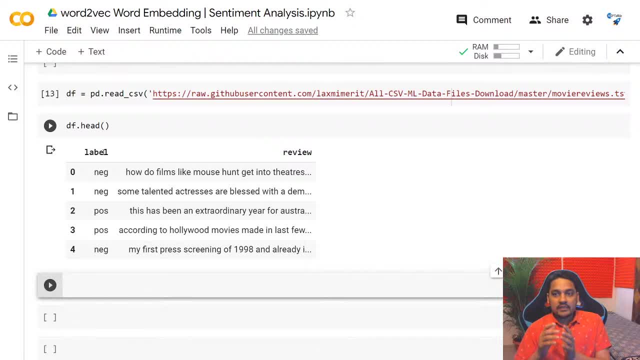 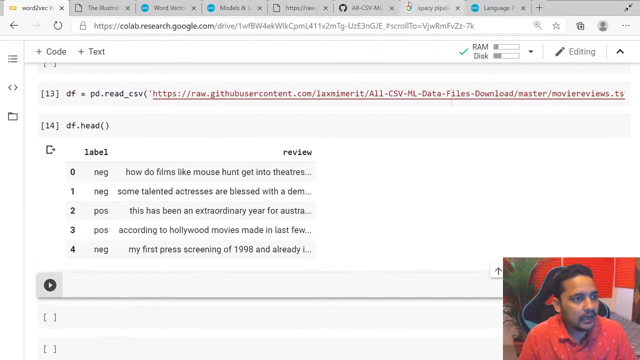 so this review is text data, so the based on this, these reviews, we will be predicting their a label which is a target variable. all right, perfect. and one more thing: we have to. we have to do, also here, a lot of processing, pre-processing. so for that pre-processing i i also have there a python. 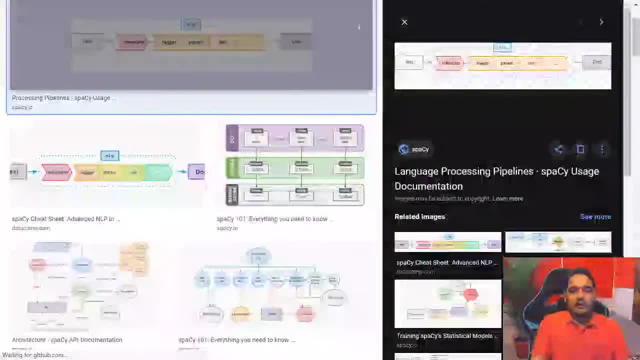 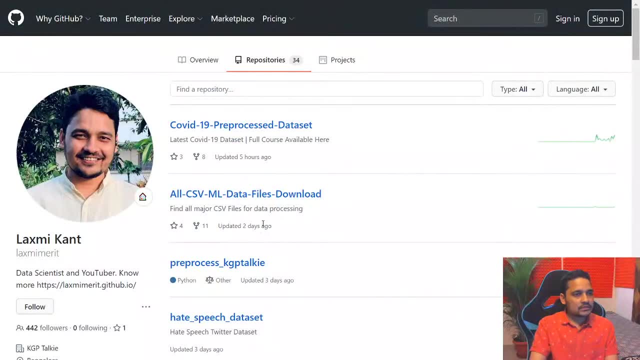 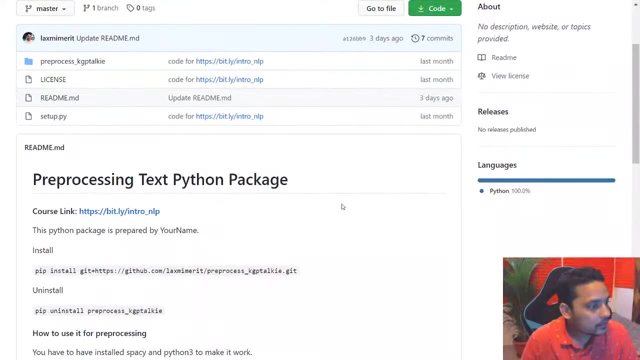 package at my github repository. if you visit at my github repository, there is a. there i have a pre-processed kgp talkie, all right. so with this pre-processed kgp talkie, you have here how you can install it. so this pre-processed package.